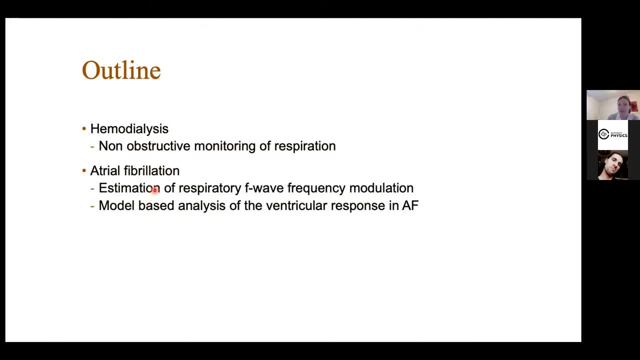 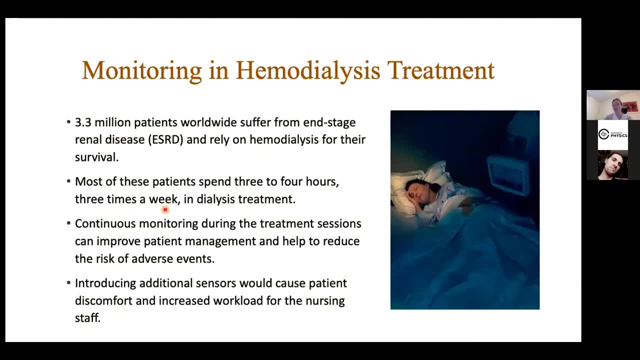 cardiac arrhythmia, And I will talk about two of my recent projects related to that. So if we start with hemodialysis and monitoring in hemodialysis, so there are quite a few people in the world that suffer from end-stage renal disease that rely on hemodialysis for. 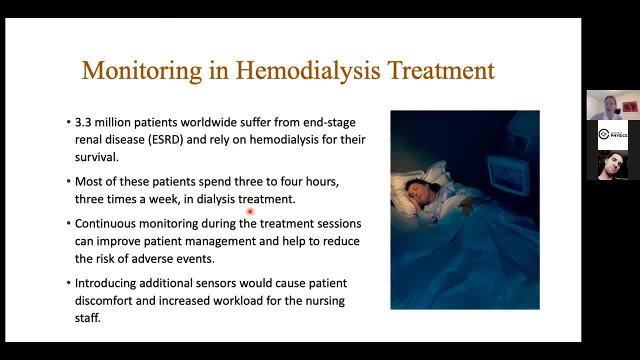 their survival. So they usually spend three or four hours three times a week in dialysis treatment, which is a lot of time, And it would be good to monitor them continuously during the dialysis treatment sessions to improve patient management and help to reduce the risk of adverse events. 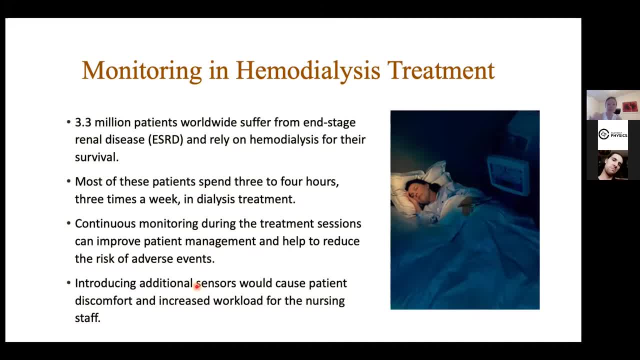 But if we introduce additional sensors such as ECG monitoring, which is a very common thing in the world, it's not going to work. So if we introduce additional sensors such as ECG monitoring or PPG monitoring, that would cause patient discomfort And it's a lot of time that the patients spend in dialysis. 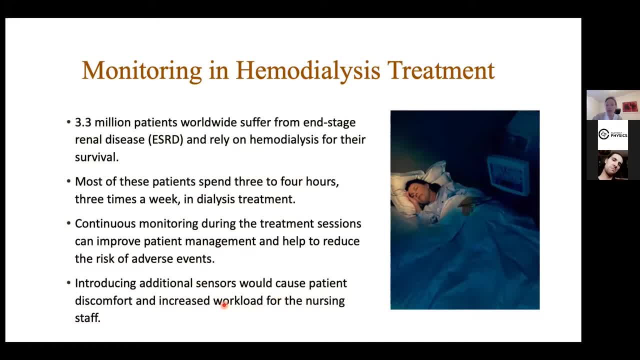 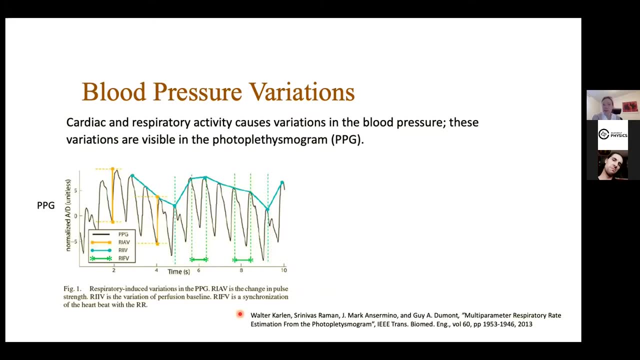 so we want to avoid this. Also, introducing additional sensors would increase the workload for the nursing staff, which would also increase the cost. So one thing that we would like to monitor is cardiac and respiration activity. Cardiac activity and respiration activity also cause variations in blood pressure. 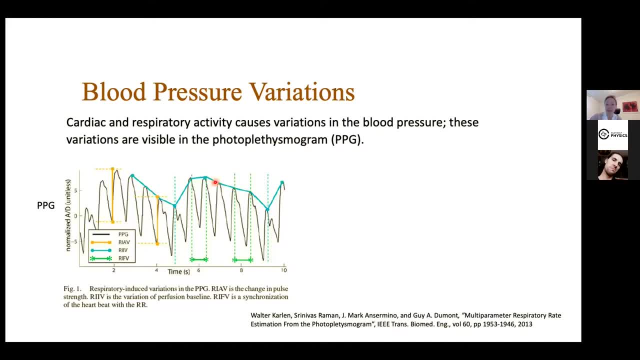 We can see, for example, from the finger PPG. so this is an example of a finger PPG signal And we can see that the blood volume causes these changes, due to the cardiac output causes this pulse pattern, amount of reflected light that varies with the blood volume in the fingertip over time. 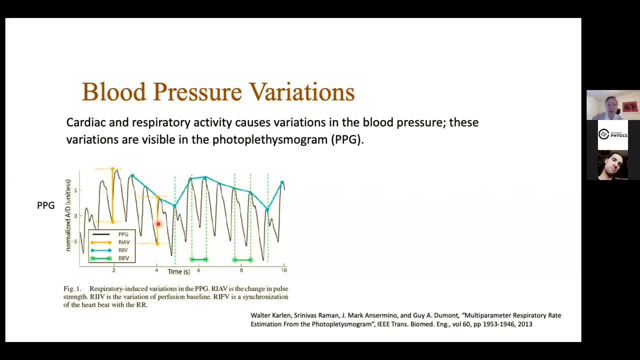 So these are the cardiac pulses, but we can also see the respiration activity, because respiration causes the magnitude of these cardiac pulses to vary over time. So with inhalation we have a slightly smaller pulse and exhalation we have a slightly larger pulse. 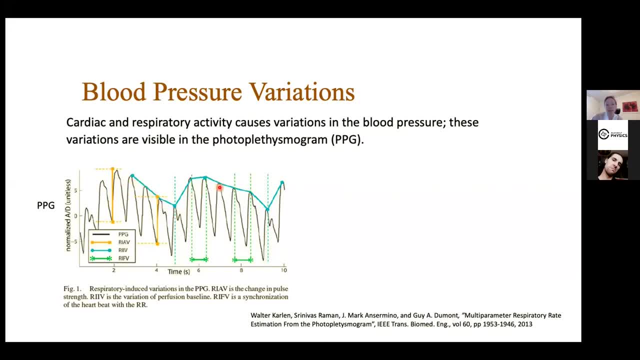 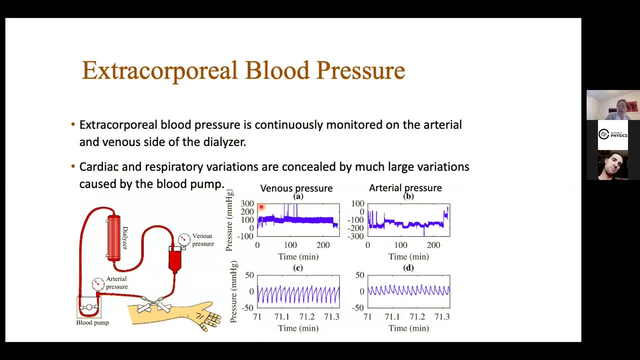 And also there is a baseline variation that's caused by changes in thoracic pressure over time, induced by the respiratory movement, And what we would like to do is to measure these variations in blood volume directly from the pressure sensors of the dialysis machine. So in the dialysis machine, 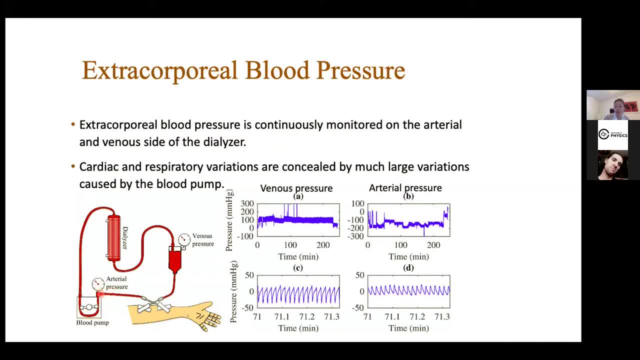 there are two pressure sensors, one on the arterial side and one on the venous side, And this is the signals obtained during a complete dialysis treatment for one patient. So this is a venous pressure signal and this is the corresponding arterial pressure signal. 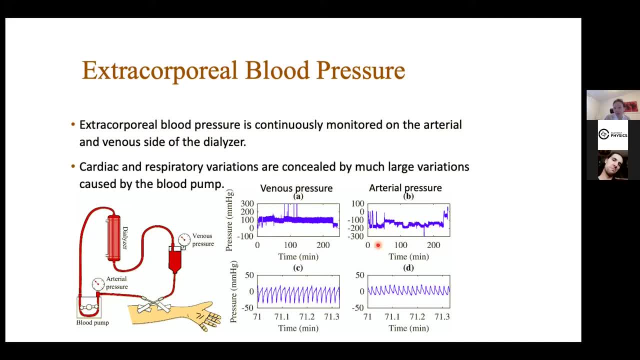 And, as you can see, there are quite a lot of disturbances. There is some baseline changes, some drift in the signal, But if we zoom in on a nice piece of the signal we can see that it looks something like this: But this is actually not the cardiac pulses. 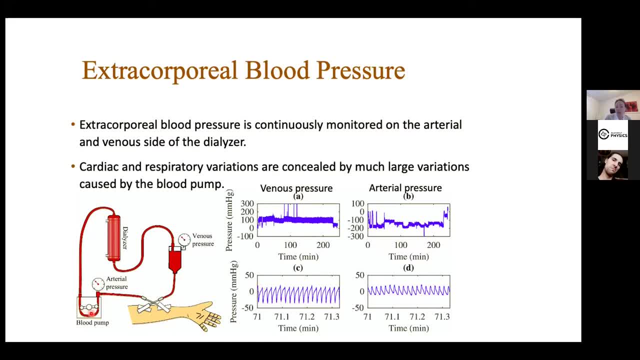 These are pulses from the blood pump of the dialysis machine. So these are the signals, these pressure signals. they contain very large pump pressure pulses And if we want to look at the small variations in the pressure signals induced by cardiac and respiratory activity, 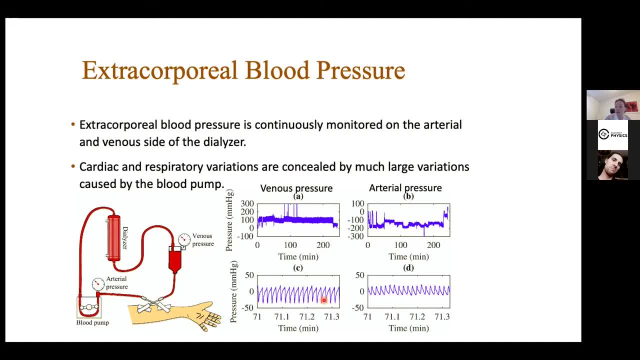 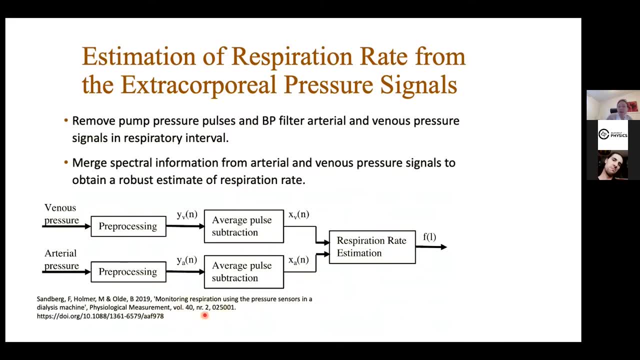 we need to remove these pulses. So this is what we are trying to do, So this is what we did in this work. Following pre-processing, we subtract average pressure pulses related to the blood pump of the dialysis machine And once we have done that, we filter the signal in the 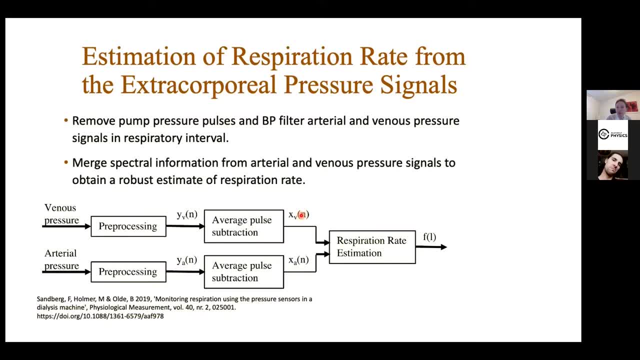 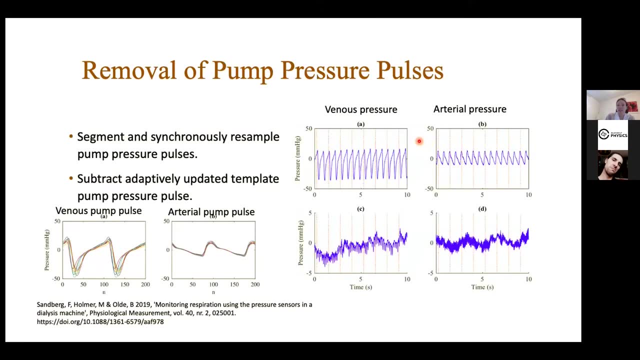 respiratory interval, so within the respiratory frequencies, And then we, based on these signals, we aim to estimate the respiration rate. So this is an example here. This is a zoomed in segment: 10 seconds of the venous- no, sorry, 10 minutes of the venous pressure pulse, And this 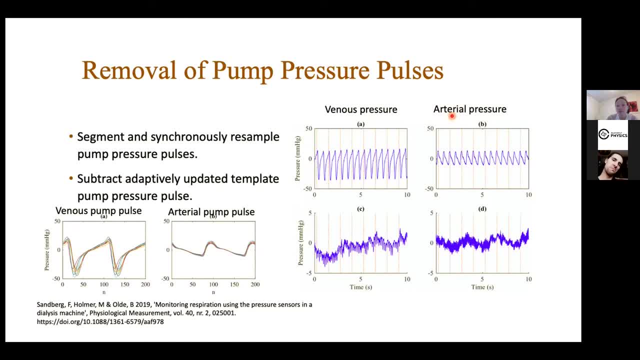 is on the right side, it's the arterial pressure, And since the magnitude of these pump pulses are so large, also minor variation in the pump pulses will be much larger than the variation induced by respiration and cardiac activity. So we need to make sure that the subtraction of the 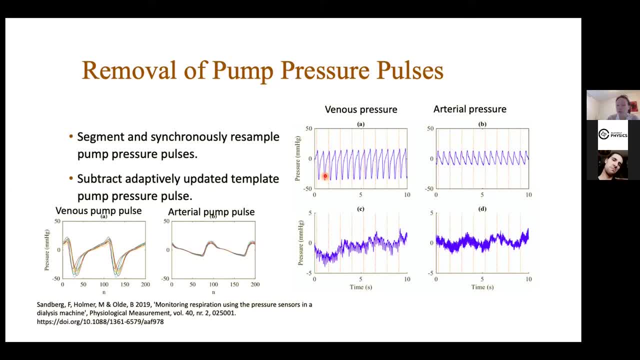 pump pulses is with a very good fit. So, in order to do so, we resample the template pump pressure pulse based on this. so there is a, simply a sample of the pressure pulse, And based on there is a. there is a sensor in the dialysis machine. 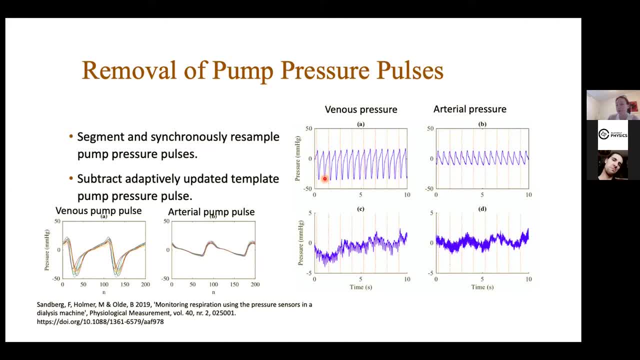 so you know in which stage the blood pump is in. So based on that information we can resample the signal. And so we got a synchronously sampled pump pressure pulse. And then we subtract this from each pressure pulse in the pressure signal. 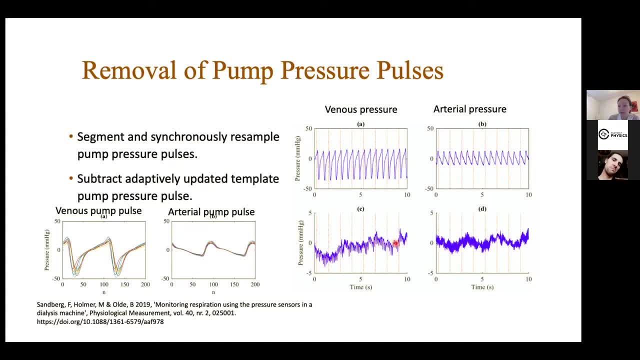 So this is the original signal and this below is when we have subtracted and the fitted corresponding pump pulses. So in this signals on the lower panels is the respiratory and cardiac activity variations in the pressure pulse And this as you can see the magnitude of this. 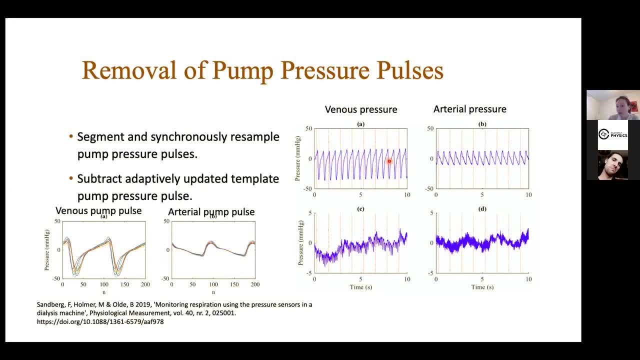 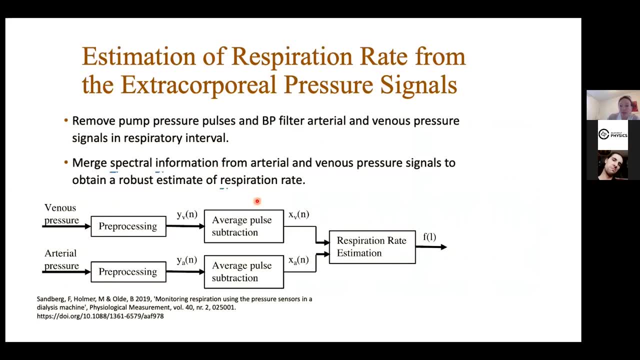 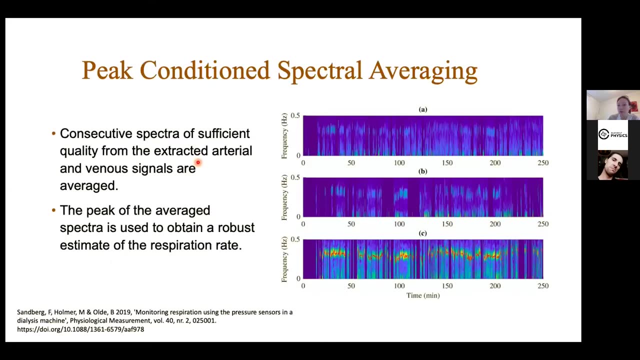 are much smaller than the magnitude of the pump pulse. So that means that the pressure pulses are much bigger than the pressure pulses. Okay, so once we have these signals, we want to estimate the respiration rate, And in order to do so, we merge the spectrum. 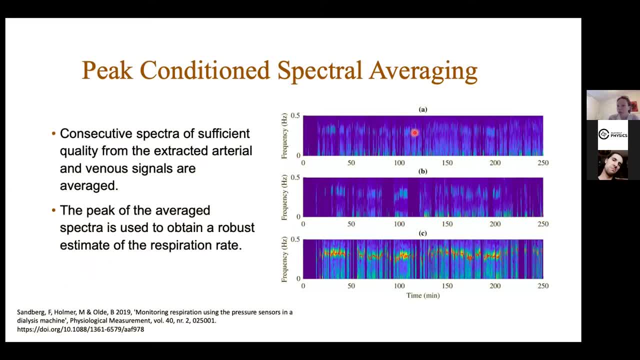 of the two signals. So on the upper panel here is a spectrum from the venous pressure pulses panel is the corresponding arterial and the spectrum of the corresponding arterial signal. And what we do is, for each time instance, we average the spectra and we also have a quality. 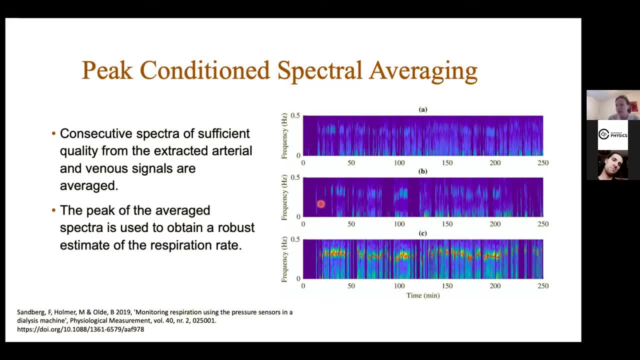 control to see that the spectra actually contains respiratory activity, and based on that we get an average spectra and from this average spectra we estimate the respiration rate. So it's a way of merging information in these two signals to produce a more robust estimate of the respiration rate. So on the lower panel, here it's the average spectra and the red. 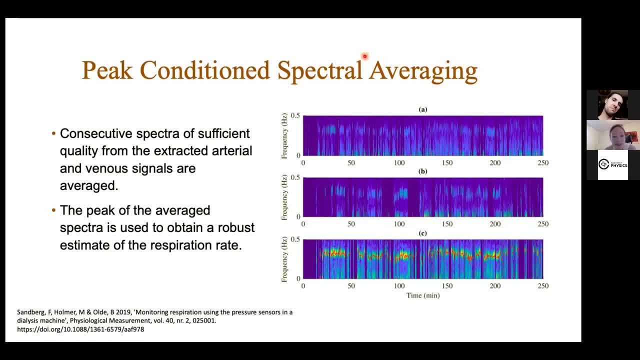 line here. Yes, I have. I think I got a question. Sorry, I raised my hand. I was wondering: why do you think that's important? Why do you have such gaps in the time of the sampling Here, Yeah, here, and say around 100 minutes? So there are gaps, yeah. 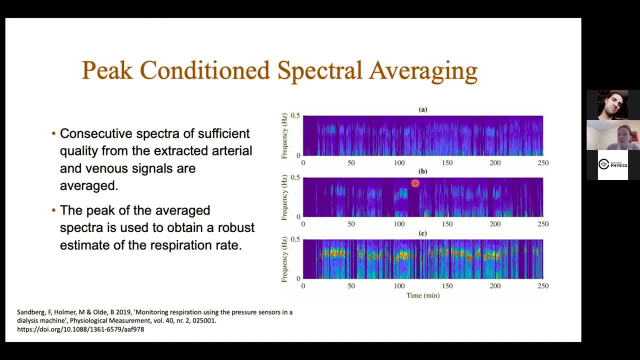 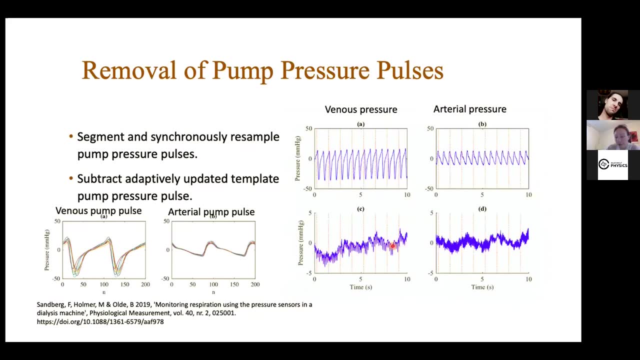 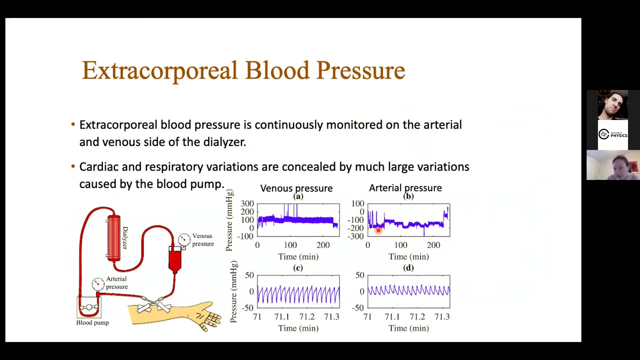 Yes, yes, And that's because the signal is the spectra, is not considered of sufficient quality. So the signals that we extract here, the filtered, once they are filtered they may contain, in certain parts they may contain large artifacts, like for example here: in the original signal there is there are quite large noise in. 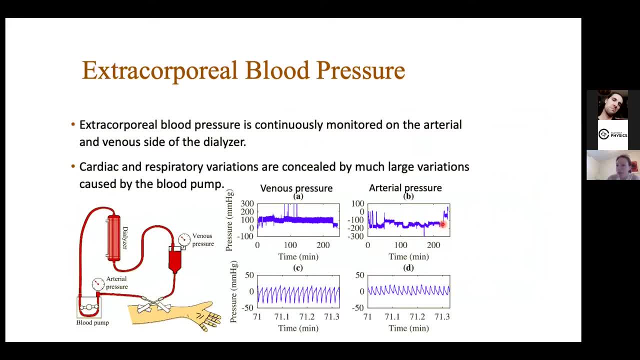 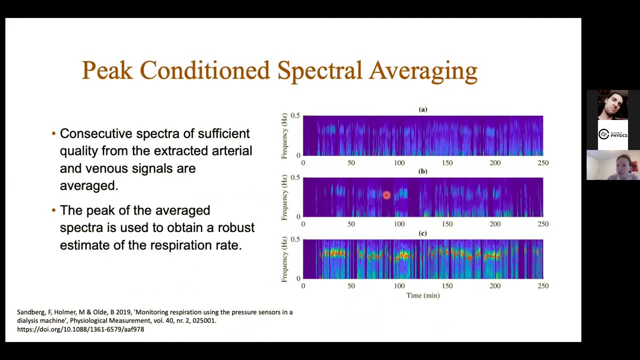 some parts of the signal and we want to make sure that that noise is not propagating to our respiration rate estimate. So therefore it's there is a quality control. So we only include those spectra that have a peak of sufficient size in the respiratory interval And those that have 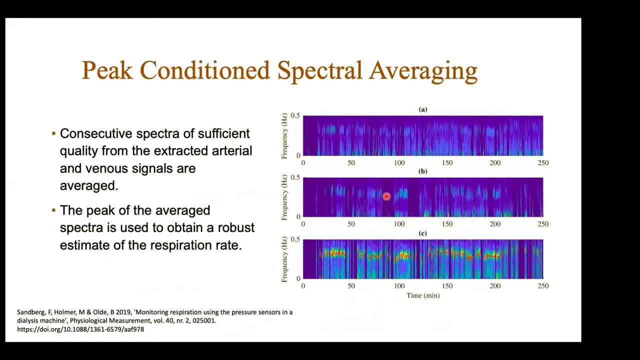 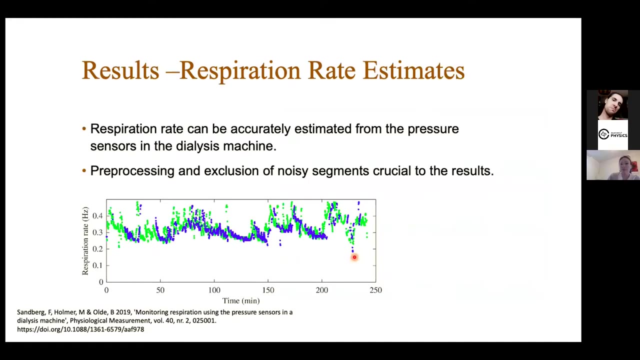 most of the spectral content in other parts of the spectra are considered as too noisy to be reliable to use for estimation of the respiration rate. So it's a type of quality control in order to Okay. thank you, Yes, So if we look at this. so this is an example from one patient during a complete dialysis. 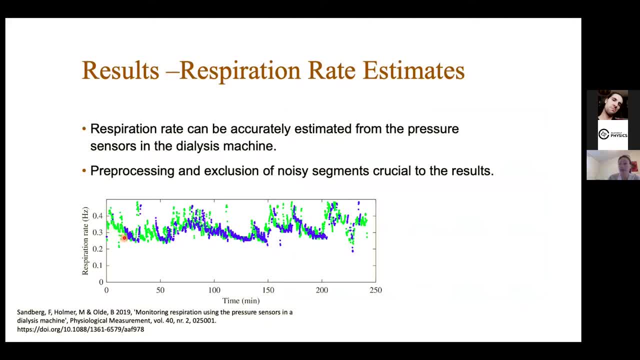 treatment And this patient, he had a CAPNO. so reference respiration signal And the reference respiration rate is the green dots here. So that's as estimated from the reference CAPNO signal. Okay, so Okay. And the blue line here, or the blue dots, are estimated from the extracted pressure. 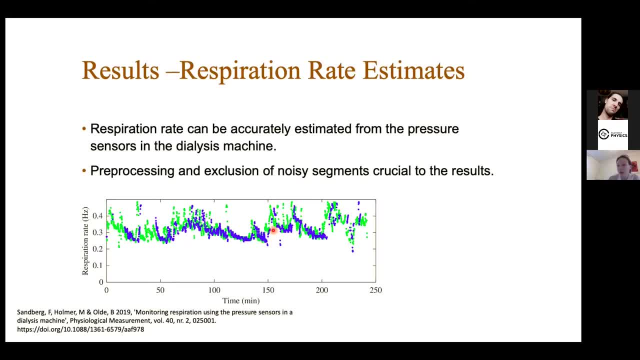 signals, respiration signals from the pressure of the dialysis machine. And here we can see that where we get an estimate of the respiration rate, it's accurate, it's fairly accurate, it's sufficiently accurate to be used for clinical purposes. 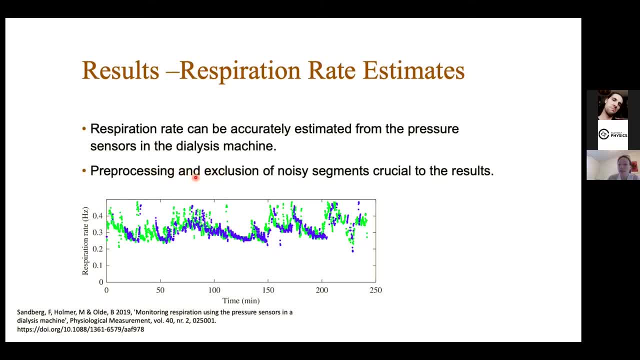 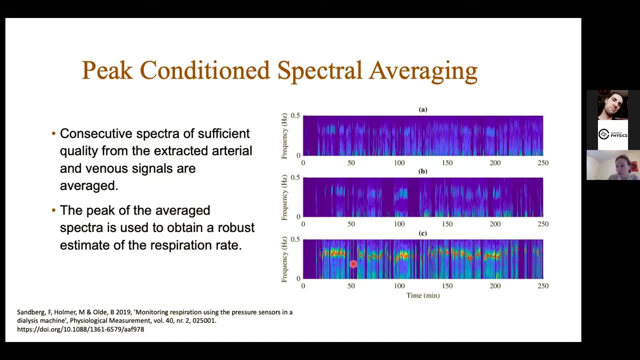 But what's important to note here is that this exclusion of noisy segments and quality control is crucial to the result. So, for example, if we didn't have this type of quality control here, we would probably get an erroneous estimate of the respiration rate in this interval. 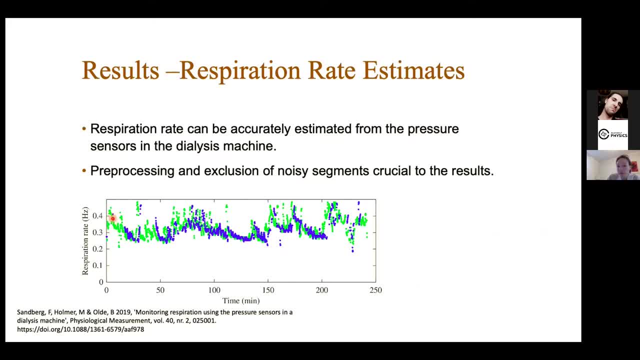 And then it's better to say that it's not possible to estimate the respiration rate. So, rather than presenting an inaccurate respiration rate, it's better to say that it's not possible to estimate it in this segment. Yes, Sorry again, I was just wondering what is the sampling rate of those pressures? 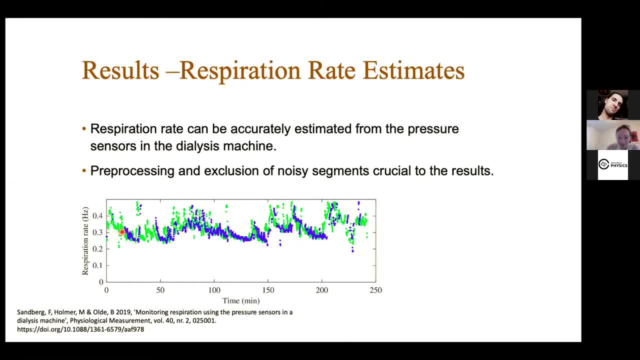 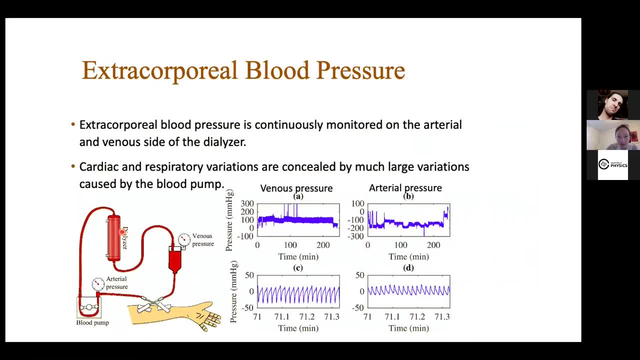 Because the time, The time scale here is in minutes, and how often do you sample those? So the original pressure signal, this one, is sampled at, I think, one kilohertz. so it's quite high sampling rate, Oh yeah. 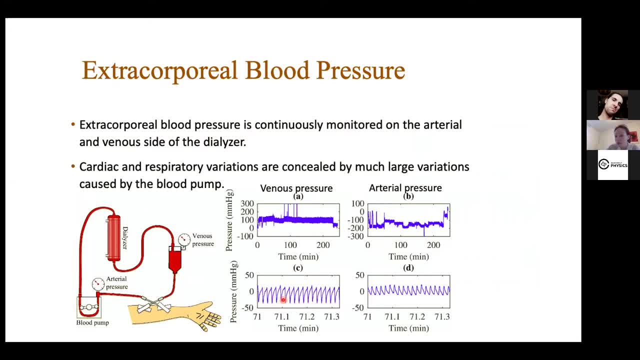 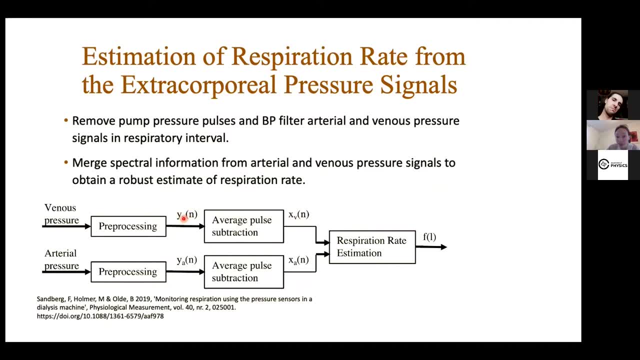 Yes, So the original signal and that's also needed in order for accurate removal of these pressure pulses. So the sampling rate here is quite high Here and for the average pulse subtraction, Whereas once we have subtracted the respiration rate or the respiration signal, here we don't. 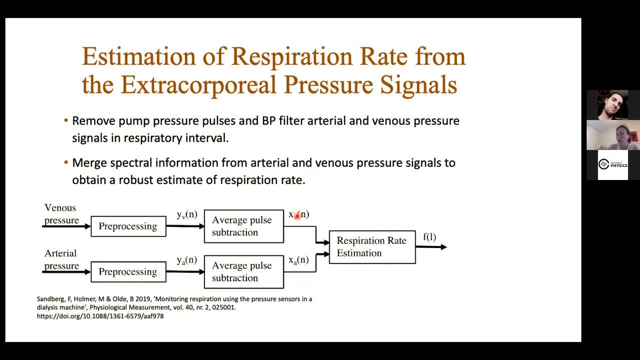 need as high sampling rate, because the respiratory information is- I mean the respiration rate- is between 0.1 and maybe 0.4 hertz or so, so there is no need for a very high sampling rate here. Mm-hmm. 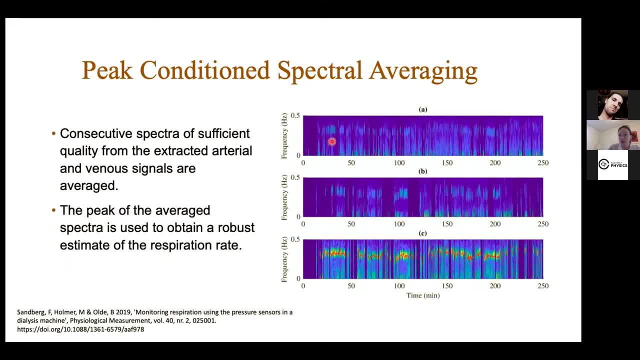 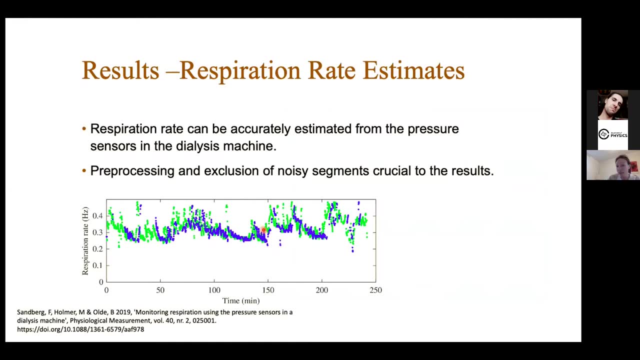 Okay, Okay, thank you, Yeah. And then, of course, in order to estimate the respiration rate accurately, we need a fairly long segment, and that's why we can't get an extremely high resolution for the respiration rate estimation here. 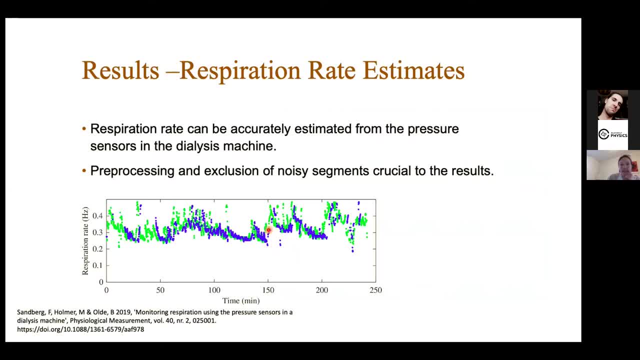 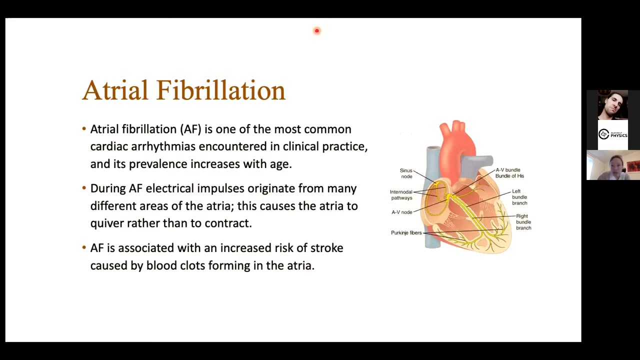 Yes, And so any more questions about this? No, Okay, No. So this was just one example of a project that I've been working with recently related to cardiovascular signal processing and hemodialysis. Okay, I think We have a question from the chat. 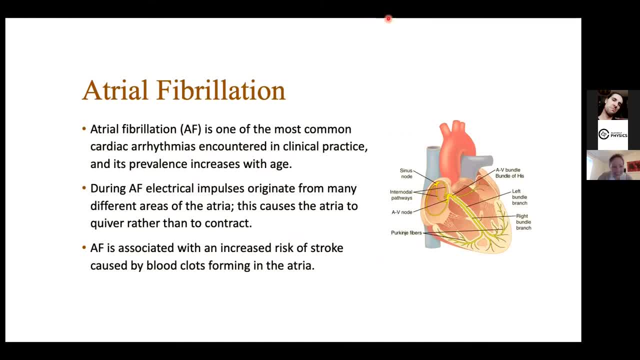 Yes, Let me see if I can get access to the chat. I don't see it. I will read it. Okay, Perfect, Yeah, So why not just take average or variance of signal with pump machine and consider resulting curve for respiration estimates? 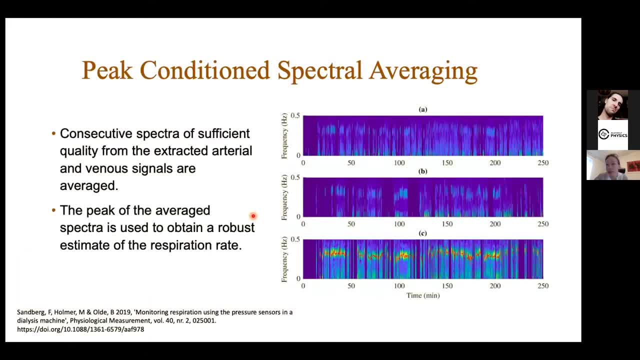 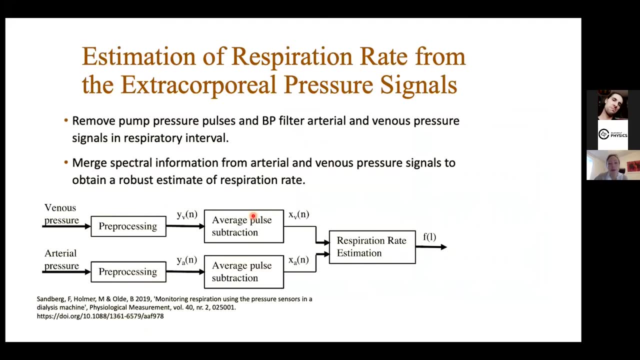 Can you say that again? I think I missed, Sorry. Why not just take average or variance of signal with pump machine and consider resulting curve for respiration estimates? The average of which signal of the original signal? Denis, could you please be more specific? 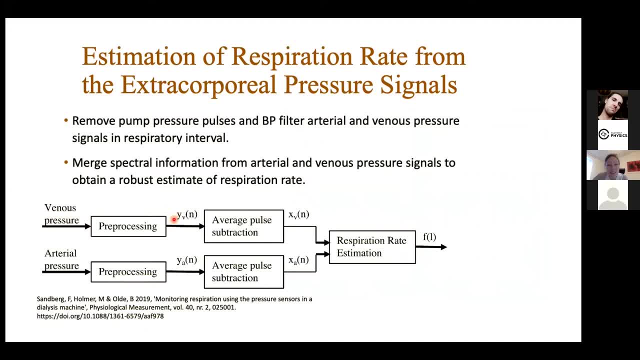 I'm sorry, I can't hear you. Yeah, let's go back to the one you said. Yes once again. OK, I think he'll write again this question. So you have on the bottom the chat or you can ALP plus H to open it. 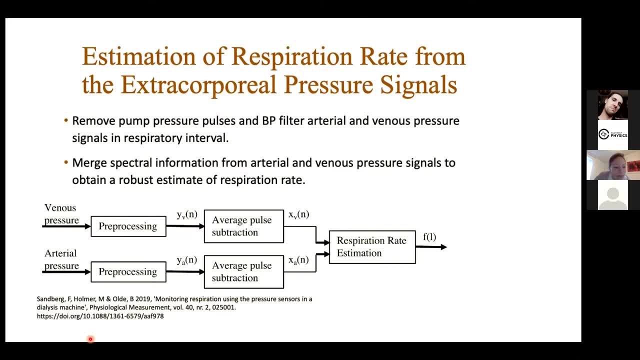 OK, yeah, OK, it's just that it's not working with a laser pointer. I just need to. OK, Why not? Why not just take average or variance of signal with pump machine and consider resulting curve? I'm not sure I understand the question. 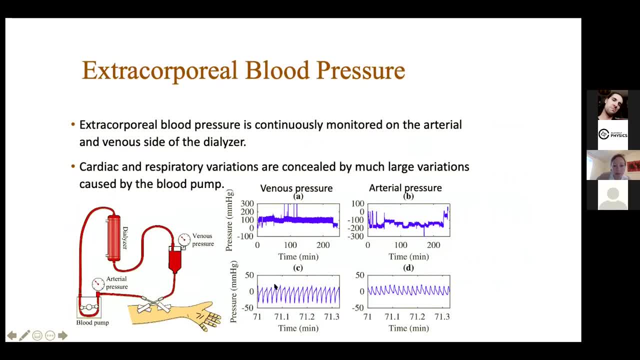 So the original signal that we observe here contains very large pump pressure pulses And we have to remove them. if we don't remove them very accurately, Also, the variations or minor changes related to changes in the speed of the pump will propagate and destroy the estimate of the respiration. 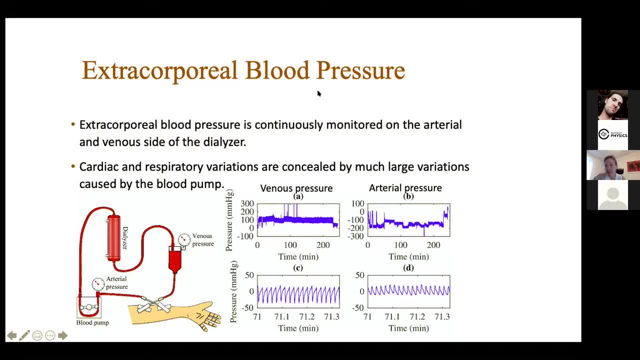 rate. I'm not sure I completely understand the question. which which average are you referring to? So I think you can move on and Dennis will rewrite his question. OK, OK, So let's continue. OK, so I thought I would go into another area where I've also 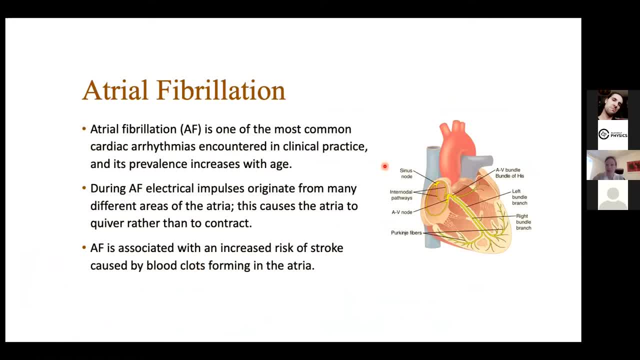 OK, so I thought I would go into another area where I've also. OK, so I thought I would go into another area where I've also worked quite a lot and that's related to Atrial Fibrillation and that's related to Atrial Fibrillation. 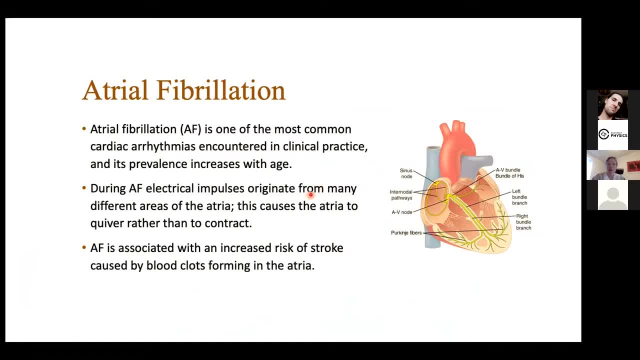 So atrial fibrillation is a very common cardiac arrhythmia and it affects 1 to 2 % of the entire adult population and its prevalence increases with increasing age. So it's very common among older patients. And if we say 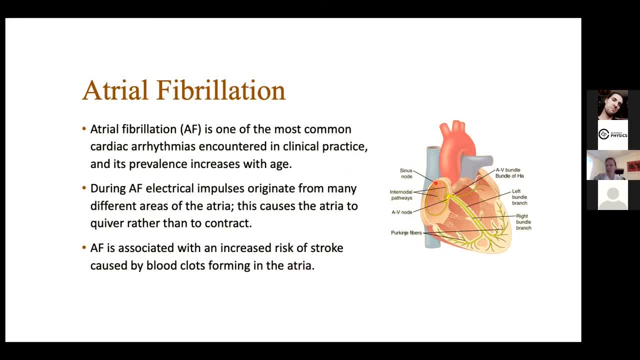 So during normal significantbehavior, this area here in the chronic laryngitis area, normal sinus rhythm- each heartbeat is initiated by an electrical impulse from the sinus node and then the electrical activity propagates through the atria, causes the atria to contract. 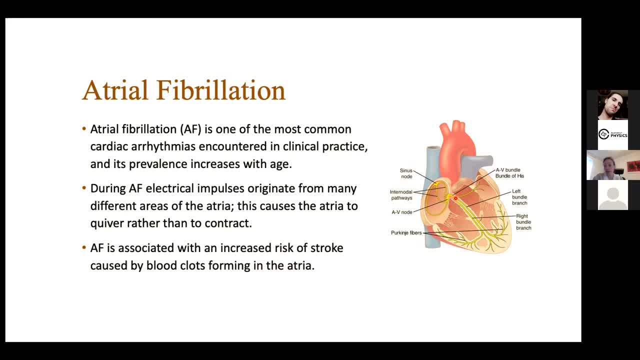 and then through the ultraventricular node, the AV node, to the ventricles and causes the ventricles to contract. But during atrial fibrillation the electrical activity in the atria is totally disorganized, so electrical impulses can start from 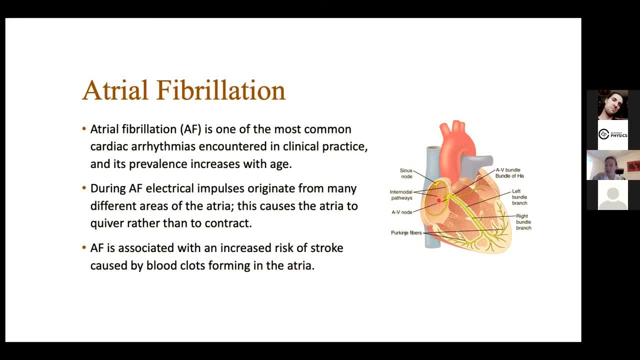 all over the atria and there are usually re-entry patterns and unorganized electrical activity and this causes the atria to quitter rather than to contract. And also because of this and the many atrial impulses arriving here, to the AV node and to the ventricles, we have a rapid and 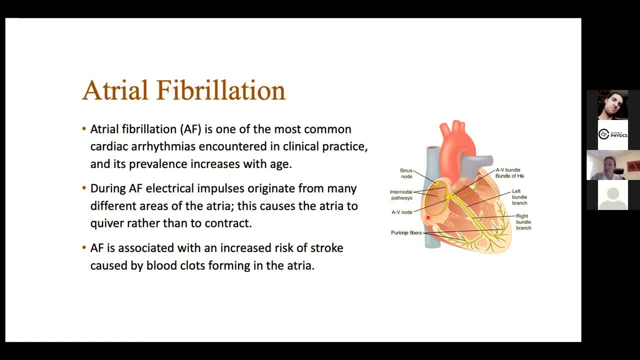 irregular heart rate. So you can live with atrial fibrillation, but it is increased. it's associated with an increased risk of stroke caused by blood clots forming in the atria. So there are several treatments, of options for atrial fibrillation. one would be to allow the atrial fibrillation to continue and try to prevent the rapid heart rates. 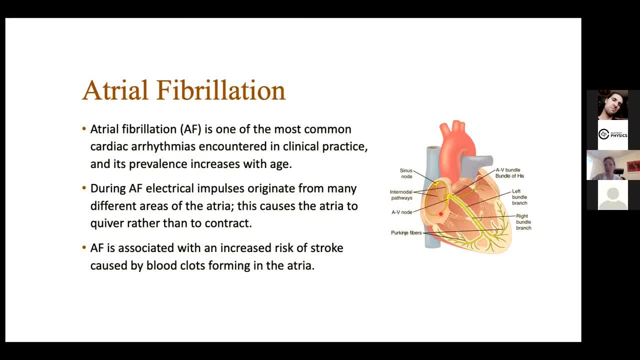 control drugs. another option would be to try to stop the atrial fibrillation and reverse to sinus rhythm, and that can be done. usually on the first first instance it's done with a electrical cardioversion, so basically an electrical shock that that puts heart back into sinus rhythm. 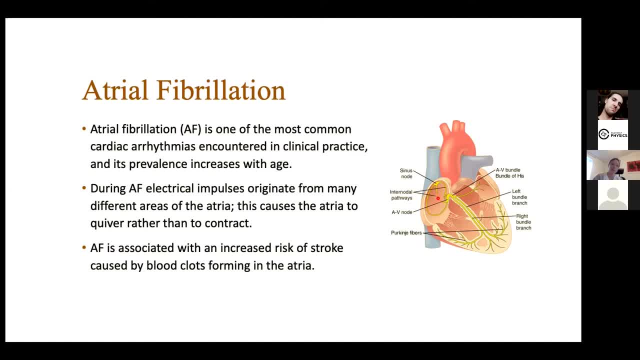 and sometimes the patient goes back into atrial fibrillation after a while. and then there are other options. there are are some, some drugs- antiarrhythmic drugs- and there is also fairly common nowadays pulmonary vein isolation, which is an ablation procedure where you go into the. 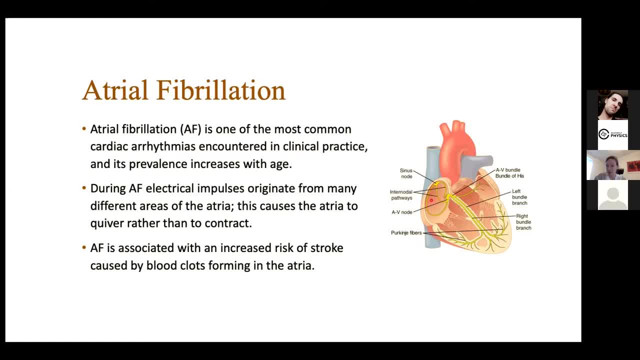 with a catheter and you burn around the pulmonary veins where there are usually triggers for this electrical atrial activity, and today we don't know which patient would benefit the best from from which treatment in advance. so it's it's. the treatment is largely based on on trial and error. 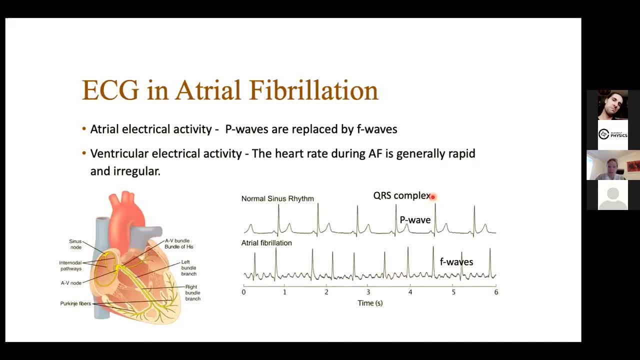 so if we look on the body surface, on the ecg, this is what an ecg looks like in normal sinus rhythm or normal heart rhythm. we have the p wave that corresponds to electrical activity in the atria. we have the qrs complex corresponding to uh. so the p wave, it's this one before, before the 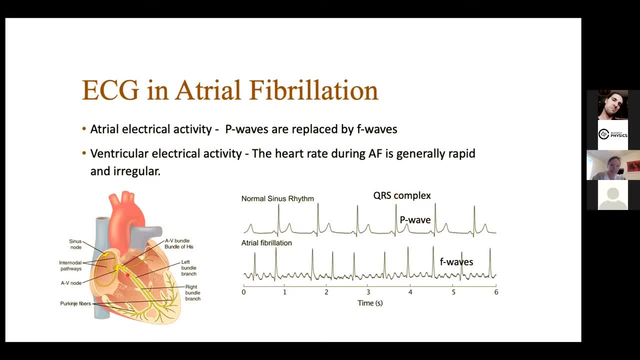 qrs complex. the qrs complex is corresponding to ventricular repolarization and uh on the panel below this is ecg during atrial fibrillation. so here we have the p waves. they are replaced by this continuous activity referred to as f waves, and that's from the continuous uh activity, of uh electrical. 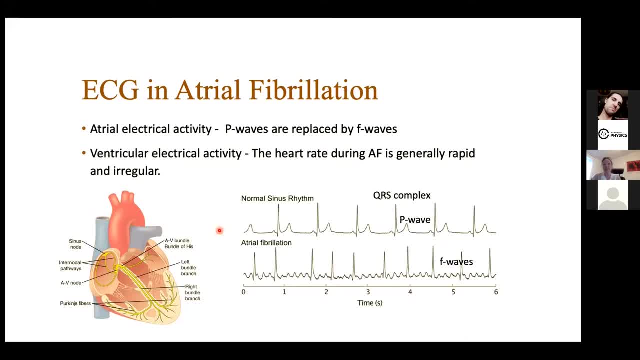 impulses in the atria and, as i said before, the heart rate. so this this is a heart rate, qrs complexes um, that's during atrial fibrillation. that's generally more rapid, as you can see here. so we have a shorter r intervals, distances between consecutive qrs complexes and also the heart rate is more. 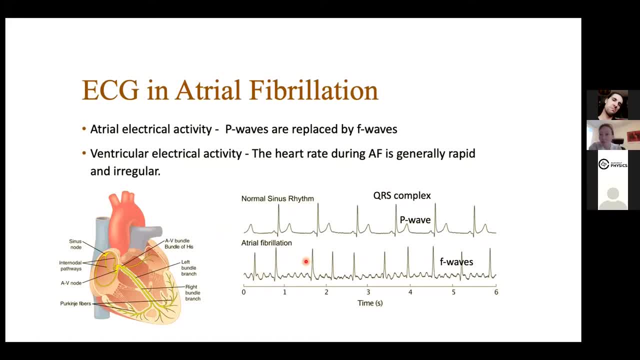 irregular. yes, uh, so sorry i have. i asked just a lot of questions. i was wondering. so the heart doesn't contract during the f waves, it only contracts during the qrs complex. right the ventricles contracts during the complex, yes, but the atria so normally during normal sinus rhythm. 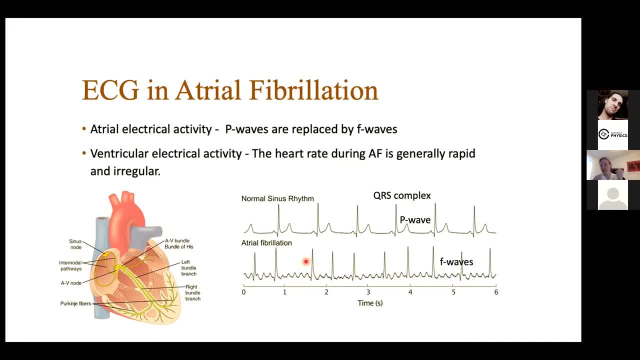 you have the filling of the atria, then contraction, and then there is a delay to allow the ventricles to fill, and then the ventricles um contract, and that those contractions, they are initiated by the electrical impulses propagating through the, the cardiac tissue. and this is the. this is what we can. 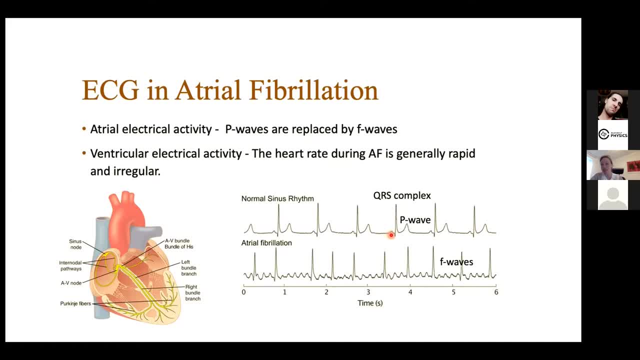 see on the body surface, resulting from that um propagation of electrical activity in the heart, but in in the, during the atrial fibrillation, the, when the qrs complex arises, uh, the ventricles do actually contract. yes, they do, they do, they do okay. and and during f wave, uh, there is what happens with the heart, with, 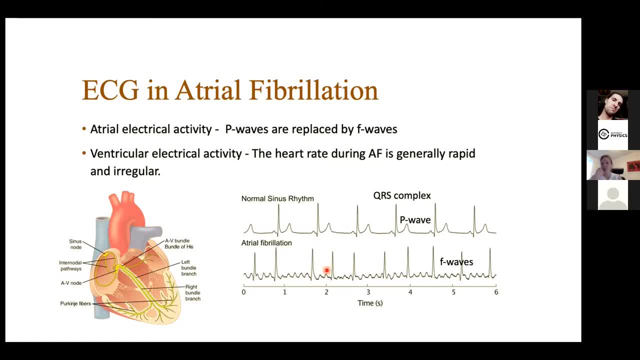 the movement of the heart during f waves, so during natural fibrillation, that the atria is is, uh, shivering, so it's less, uh, it's not pumping, it's more, it's not, and it's not completely. still, it's not like a coherent movement motion. i'm sorry, it's not like some incoherent motion in there. yes, yes, it's incoherent, it's, it's. 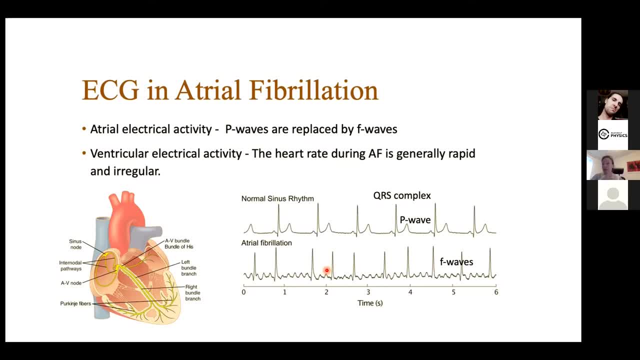 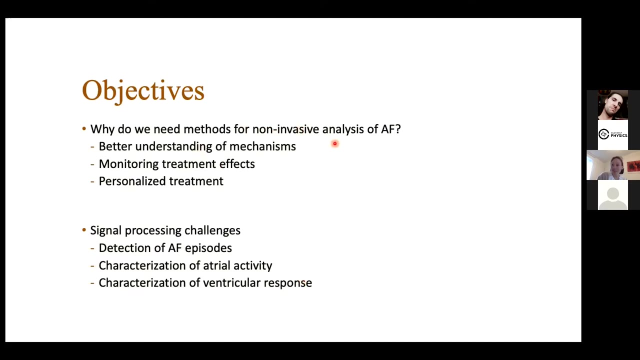 it's- uh, not synchronously, uh, pumping. it's it's more, uh, shivering, okay. okay, thank you. so the pumping function of the atria is not working during atrial fibrillation. yeah, yes, so, uh. so why do we analyze the ecg during atrial fibrillation, which is what what i'm doing and the reason why we're? 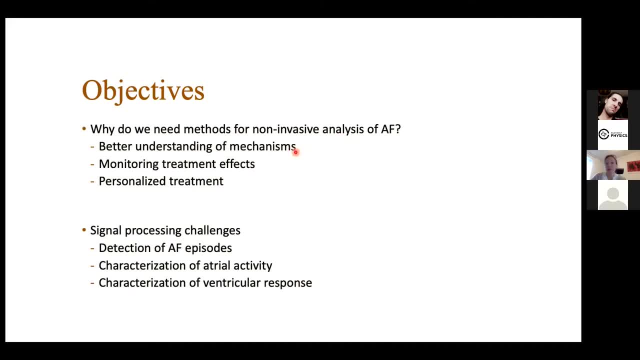 doing that and why we need methods for that, is, first of all, to better understand the mechanisms of atrial fibrillation. it's not completely known why it starts, why, why certain patients get atrial fibrillation and why others don't, and also we don't know, uh, why certain treatments work for. 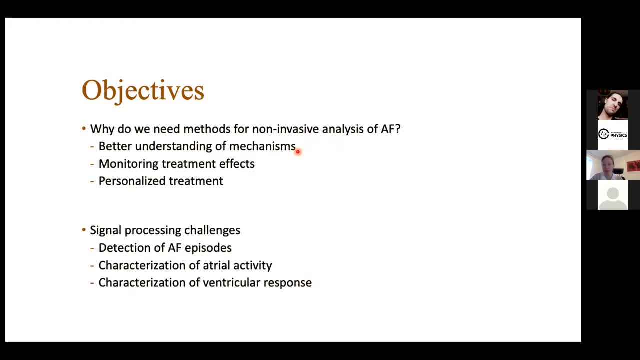 one patient and not for another. so there is um some missing knowledge here of the understanding of the mechanisms. also, it's it's would be nice to to be able to monitor treatment effects. so i mean we can, we can see if the atrial fibrillation stops or if it continues. but if you want to look at a more detailed level, 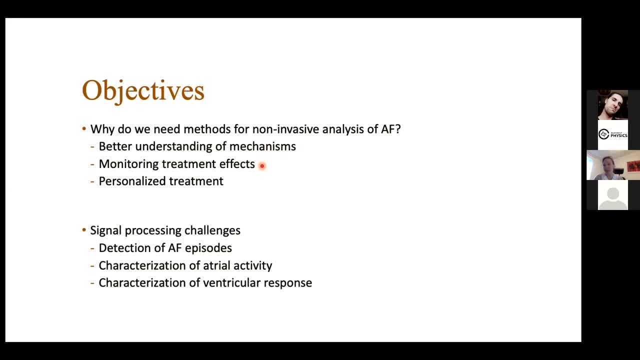 how, how does the electrical activation pattern in the atria change? or how, how does the heart rate change in response to certain treatments? we need to, we need to tailor methods for that and also, optimally, we would like to know in advance which patient would benefit from which. 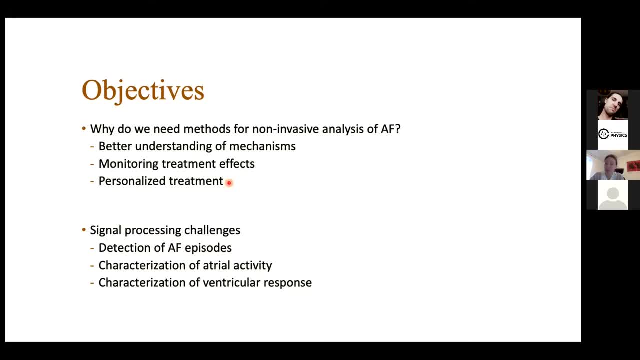 treatment. so, um for that, it would be nice to be able to predict, uh the effect of treatment. so, based on baseline characteristics of the atrial fibrillation, which treatment option would be most beneficial. so there is um quite a lot of work going on in this area. 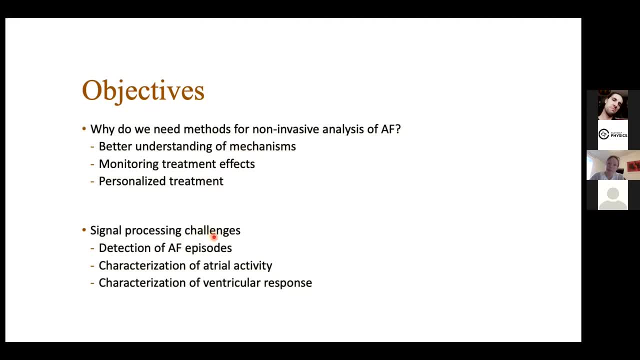 when it comes specifically to signal processing the challenges here. obviously, detection of atrial fibrillation episodes is one one, uh one one- area where there has been a lot of work done- uh of work done recently, especially related to- so we have this monitoring with the wrist watches. 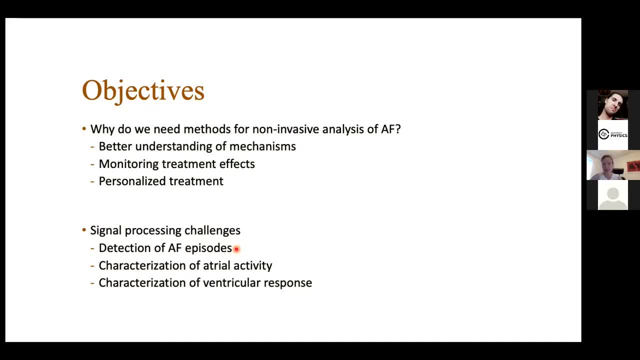 or we have other types of continuous monitoring or we have different wearables, so we want to detect atrial fibrillation in large populations. so that's one area where there's quite a lot of work going on. another area, which is what I will present more here, it's the characterization of 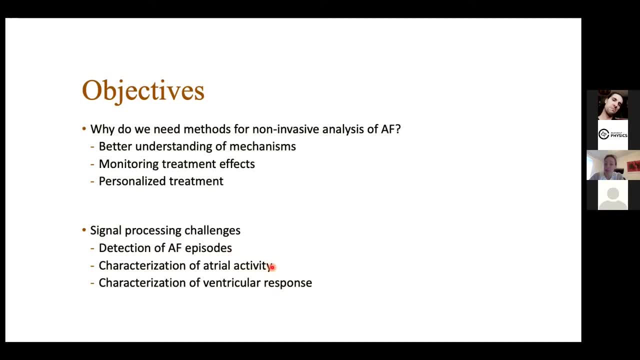 the atrial electrical activity during atrial fibrillation. so how to describe that and how is that connected to the, for example, progression of atrial fibrillation, which is related to treatment outcome? also, characterization of the ventricular response, that is, the heart rate during atrial fibrillation. how is how can we do that? what? what type of of methods can we do to? 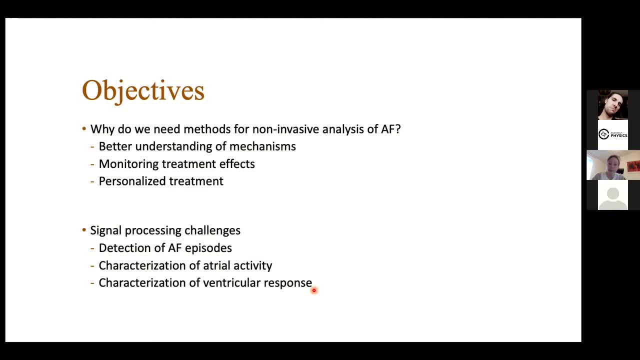 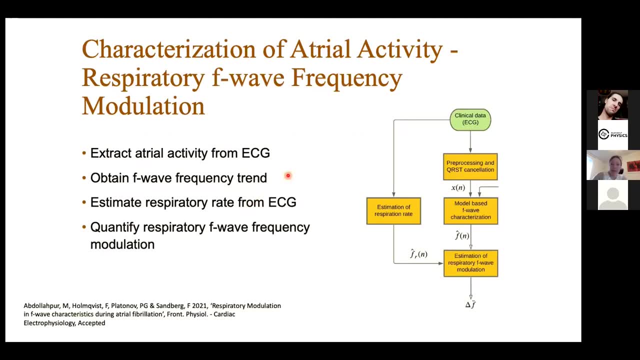 to extract relevant information from our measurements, so I will start with this. so this, this paper was actually accepted last Friday. it's fairly recent work and it's about characterization of the atrial activity and specifically looking into respiratory modulation in the f wave frequency, and in order to estimate this, there are several steps that we need to take. so we have the original. 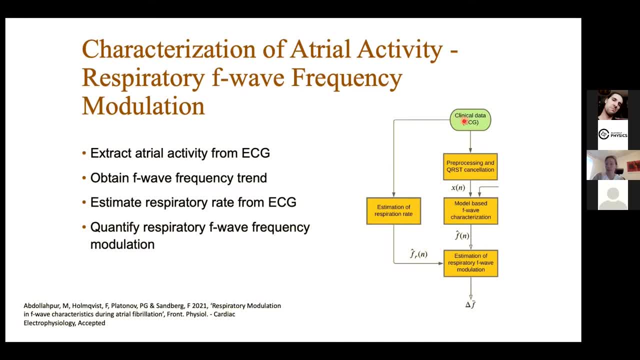 ECG and in order to characterize the atrial activity in the ECG, we first need to extract it. so we had the large QRS complex. we need to remove those in order to to analyze the atrial activity. once we have done that, we need to estimate the frequency trend. so a higher. 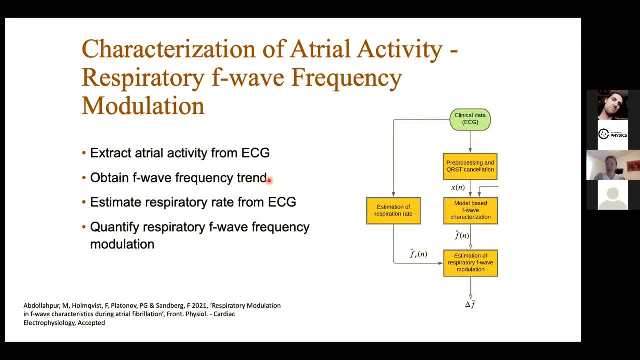 resolution accurate frequency trend. and then we need to check for modulation in the respiratory interval and to know in. to be able to do that we also would need to know the respiration rate for this patient and we can do that from the ECG. so we can estimate respiration rate from the ECG. so, looking at the frequency, 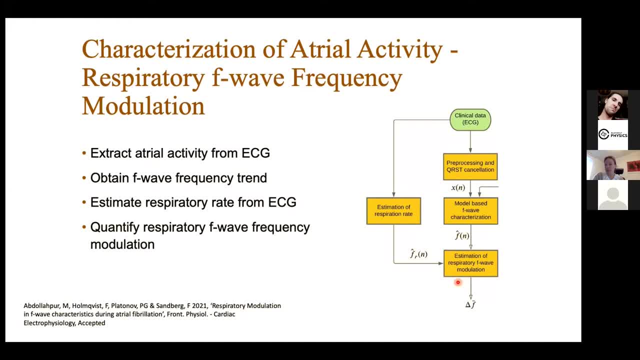 trend of the f waves and the respiration rate. we can. we can obtain and quantify the magnitude of respiratory f wave frequency modulation and this is interesting because it's linked to autonomic regulation of the autonomic nervous system and it's linked to the autonomic regulation of the autonomic 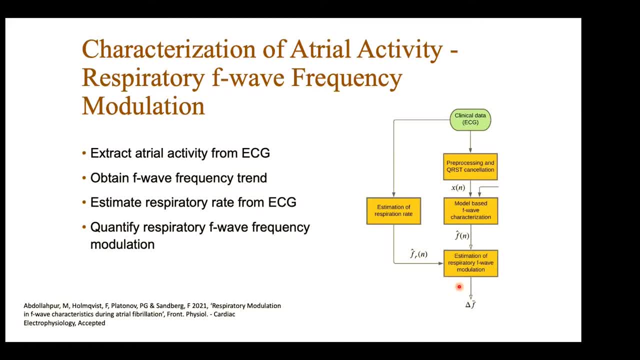 nervous system regulation of the atrial cells, and we believe that that's related to progression of the disease. so that's why we want to look into it. but it's challenging because it's it's very small variations that we are trying to quantify. so if we start with the, the first step here, 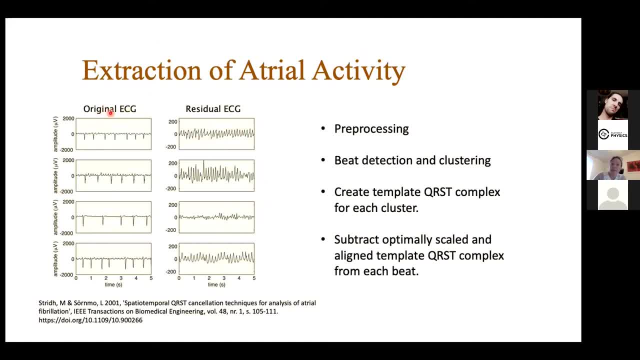 extraction of atrial activity. so we have the original ECG signal and, as you can see, the main, the main, the largest part in this signal. so these are for different examples from different patients and the largest magnitude variations is related to the ventricular activity, the QRS complex. 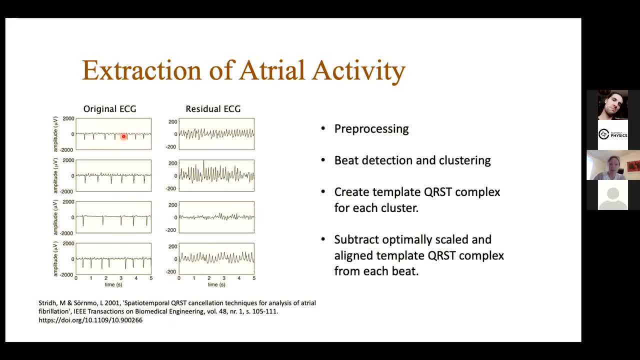 so, in order to analyze the f waves, the atrial activity, we would need to remove this ventricular activity, and there are several ways to do that. one that we have used quite a lot in Lund is to to remove an average beat. basically, we we detect the QRS complexes, that we cluster them based on 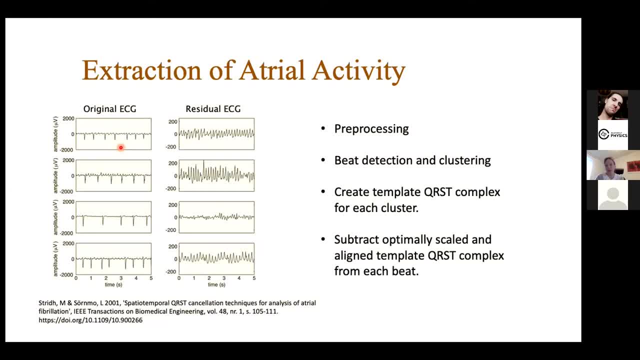 morphology. so, for example, there may be ectopic beats that have a deviating morphology and there so that we cluster them into different classes, and for each cluster we create a template which is basically the average QRS complex, and then we subtract this the corresponding template QRS. 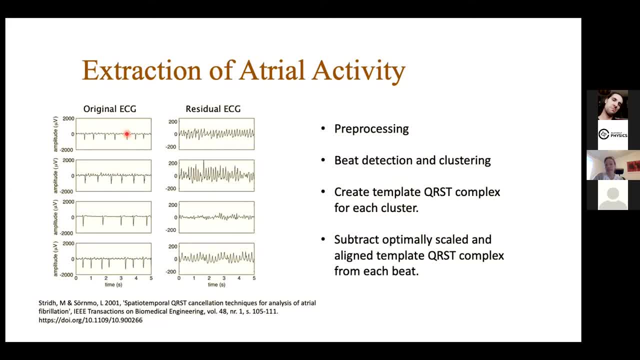 complex from each QRS complex in the signal. and when we do that, we also optimally scale and align temporally and also spatially, so distributing the, the energy, between the, the leads, and once we've done that, we obtain the, an f wave signal where the QRS complex are removed. yes, 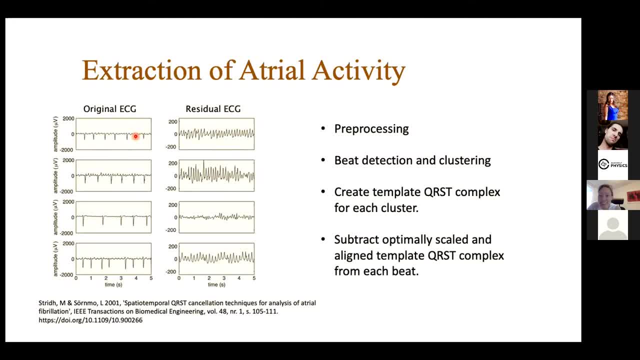 I got a question. hi, may I wonder what kind of methods do you use in order to post process this original ECG signal? post process after this removal or before removal? or yeah, yeah, exactly this process when you you remove these high peaks. yeah, in order to get residual. 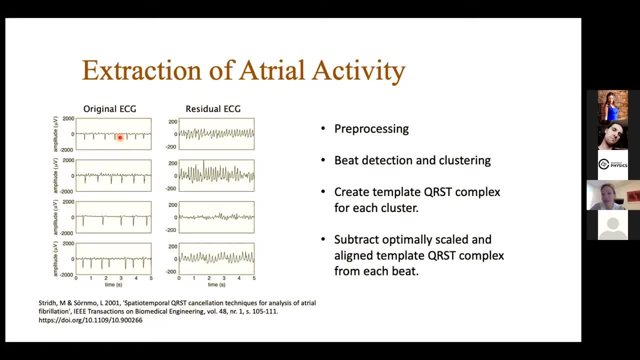 uh, ECG signal. so what kind of methods do you use? well then, the method that we used, that I used in this work, that we have used quite a lot in Lund, is this special temporal Q or SD cancellation where, as I said, where you're basically, we're basically creating a template beat, and then we are 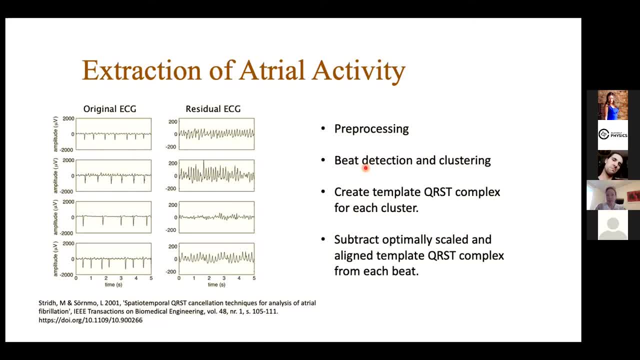 scaling, we're scaling, we're accounting for scaling and rotation of energy between leads and also time alignment. So we fit this template beat optimally to each beat of the original ECG and then subtract it basically. But there are other methods as well, I mean you could use. there have been proposals of 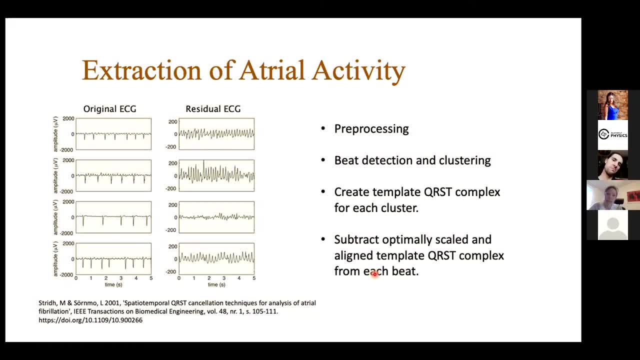 signal separation, like independent component analysis. there are actually. there has been quite a lot of work done with this, So this paper was presented already 20 years ago actually. so there are quite a few methods available for this, but this is a method that we have been using quite a lot in Lund and it's quite robust. it works in practice. 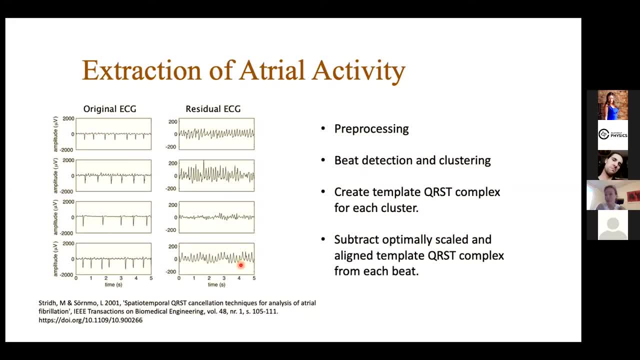 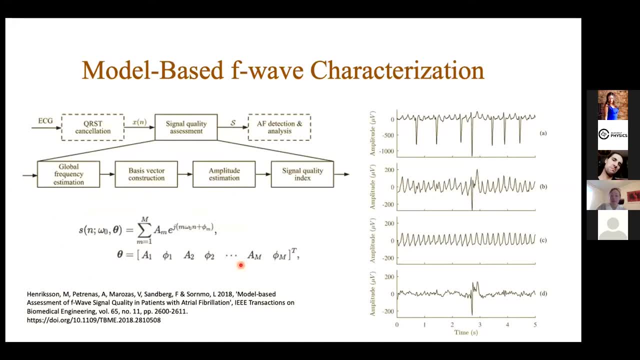 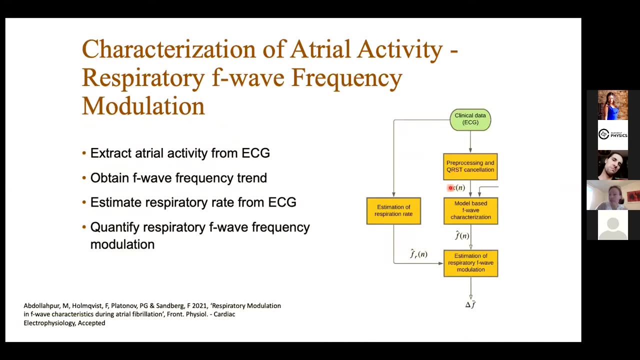 But there are other methods available. Okay, thank you, I will learn from this publication. thank you, Okay. so once we have this, once we have removed this Mehration compelc, we have the F wave signal, and then we want to estimate the frequency of the F waves. 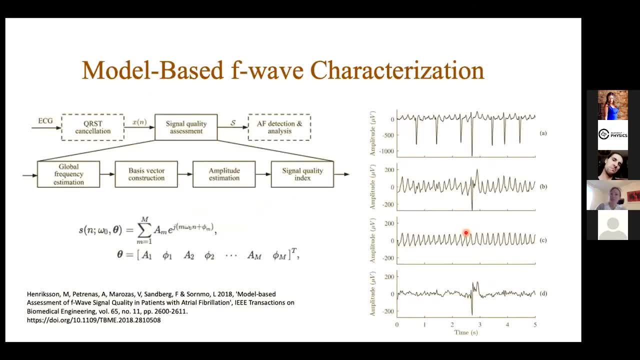 And the way we do that is using a model based F wave frequency characterisation method. So because if I want to wanted to estimate the F wave frequency of the S wave, I then need to add all of this learning that's missing in small units. 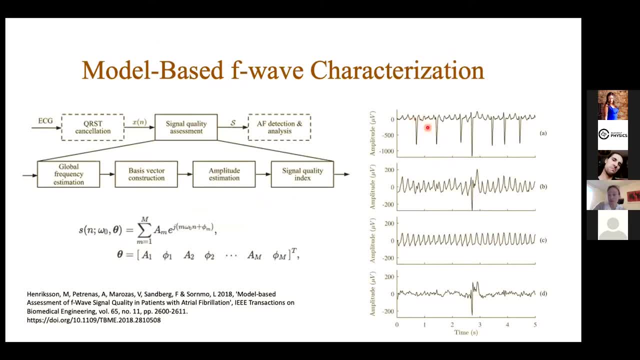 It's all going to be more complex when you're adding business-based startingAN Heav triple wave, which. So, basically, if on this right hand side panel we can see, this is the original ECG and then the next panel is extracted, F waves And, as you can see, there is some curiosity cancellation that failed. 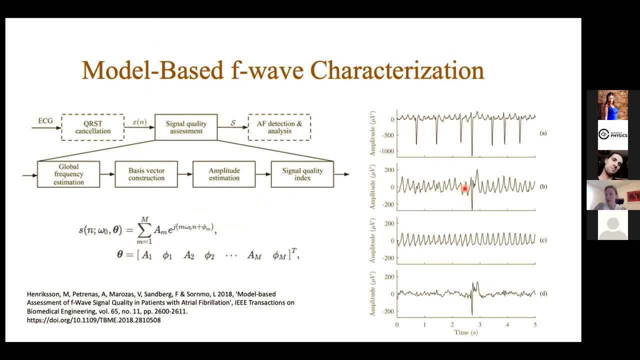 So there is some some noise, some remainders of the curiosity complex here, And also I mean this could be other types of noise as well. So sometimes there is noise in the, in the extracted F wave signal, and we want to account for this noise. 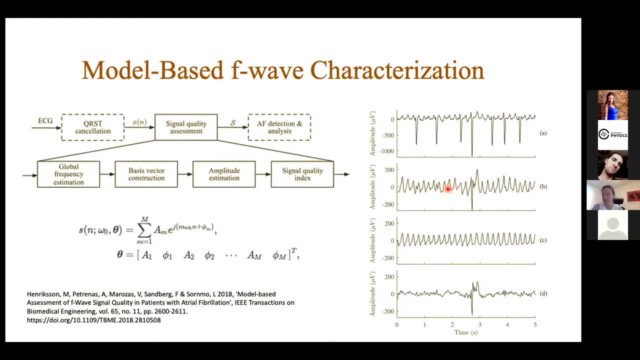 So instead of just applying a spectral analysis or time frequency analysis or so, we use a model based approach. So we fit this complex exponential model to the analytic equivalent of the F wave signal And then we look at the residual, So the difference between the fit, optimally fitted model signal and the original F wave signal. 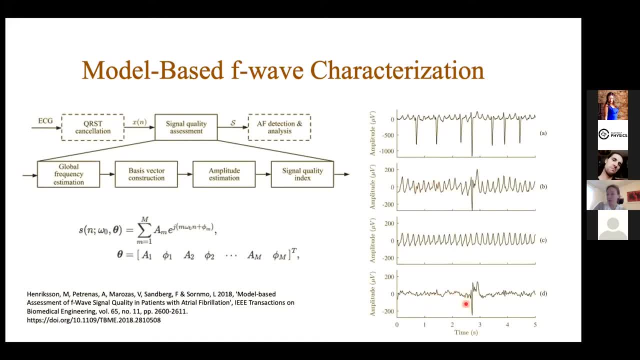 And when the difference, when the residual, is large, this is a sign that the estimates or this model parameters of the fitted model are not reliable. So we use this residual to quantify the signal quality with the signal quality And then we look at the energy index. 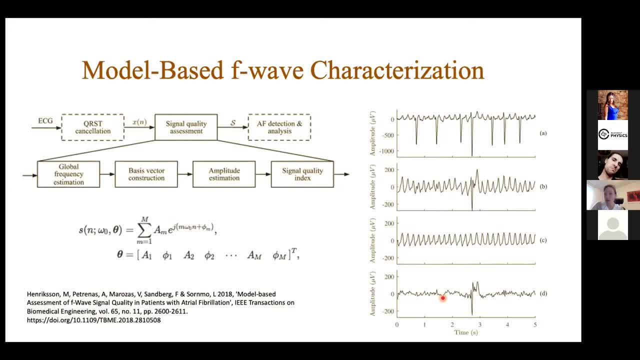 That's basically the energy in the residual signal over the energy in the original signal. So with this approach we get an estimate of the frequency of the F wave frequency, the local F wave frequency and also actually of the amplitude on the phase. But here in this work we're mainly interested in the local F wave frequency. 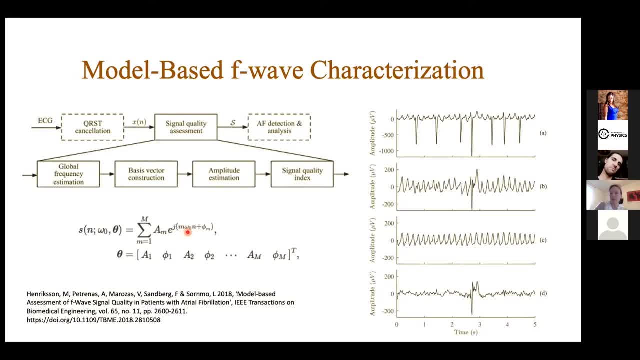 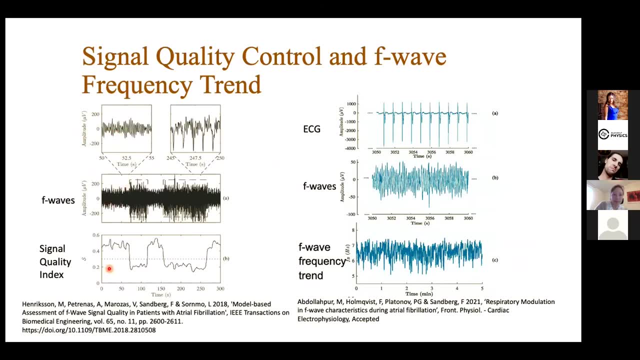 So we get a high resolution F wave frequency trend. So this is an example. This is an example of the signal quality index. So here we have 300 seconds of F waves And if we zoom in in certain areas we can see that here, for example, the signal quality is quite nice. 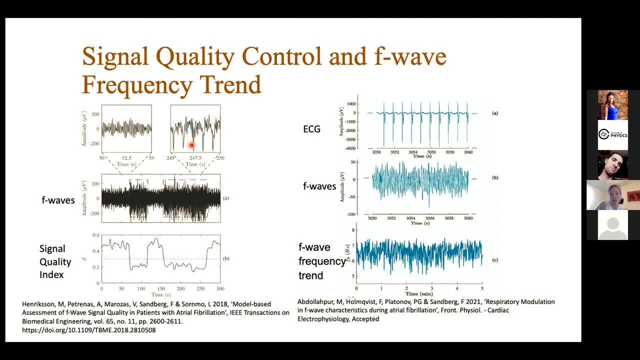 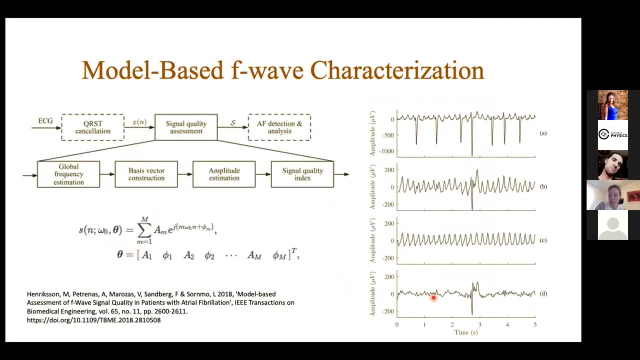 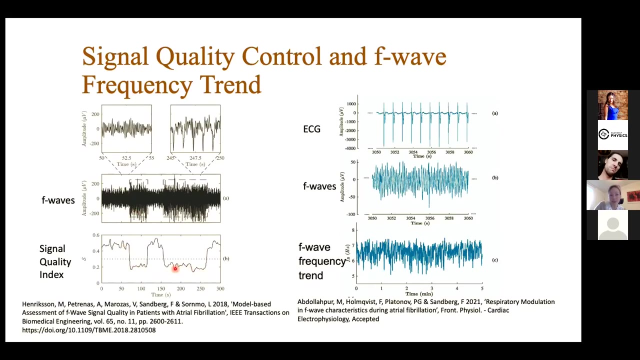 But in this area there are quite a lot of residuals. There are quite a lot of residual QST complexes where the QST cancellation failed or where there are other problems. And if we look at the signal quality index that I described here before that is based on the residual signal, we can see that the signal quality index is much lower in these areas. 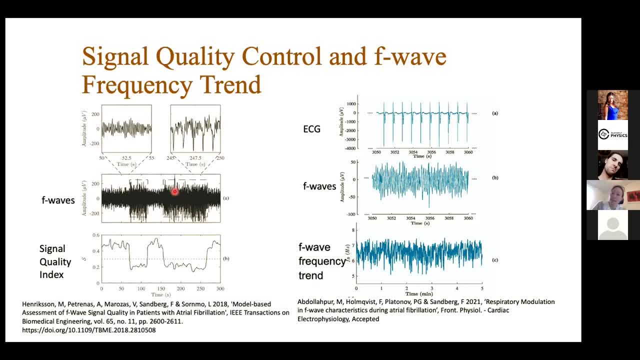 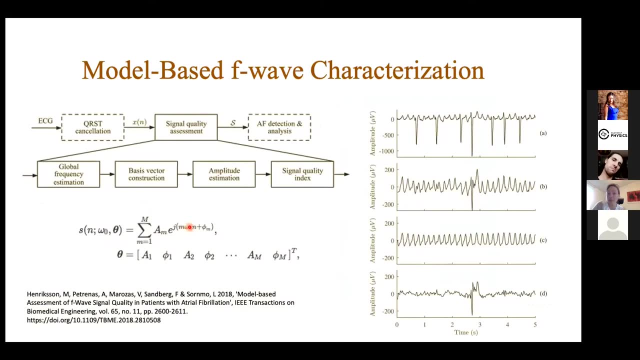 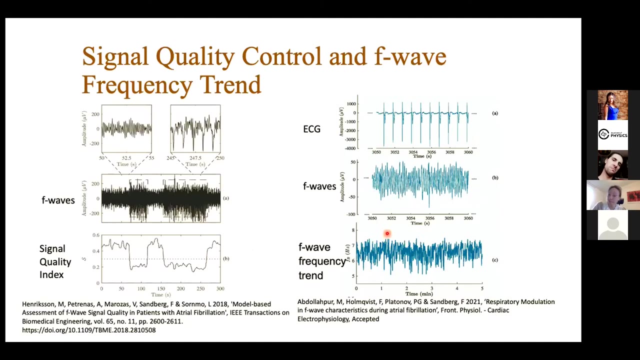 So we can use this signal quality index to determine if the estimates Are reliable. So if the model fit, If the model fit is good enough, we assume that the estimates, that is, the model parameters, are reliable. And we apply this to analyze our F waves here in the work where we try to determine respiratory modulation in the F wave frequency. 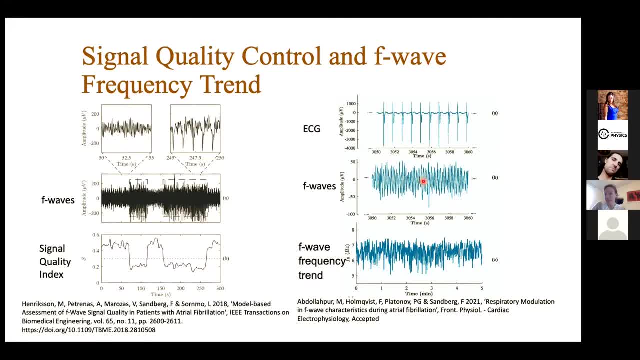 So this is the original ECG. again This is the original ECG. This is extracted F waves And then we from this, by this model fitting approach, we obtain a high resolution F wave frequency trend. So this is the frequency, the local frequency of F waves. 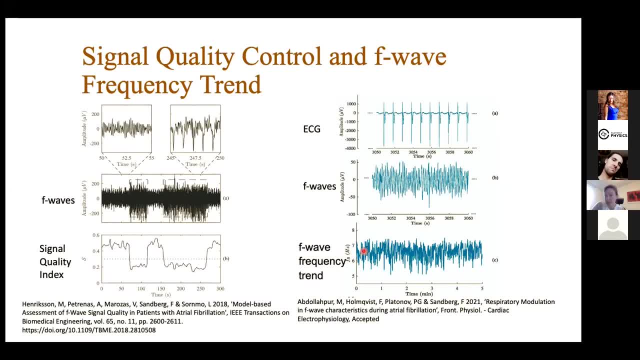 Over time. So this is for five minutes And here you can see that it varies quite a lot over time between six, seven hertz, also almost down to five hertz. So there is quite a lot of time variation And we think that, or some of this variation is related to respiratory modulation. 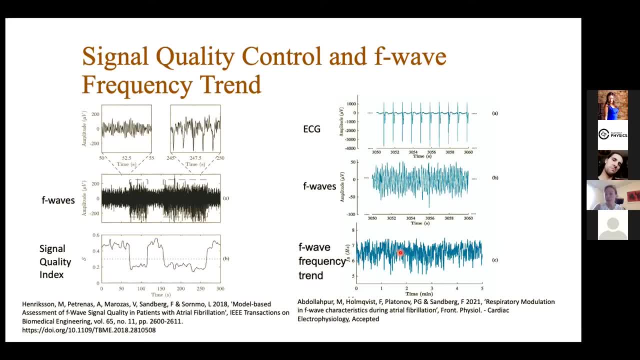 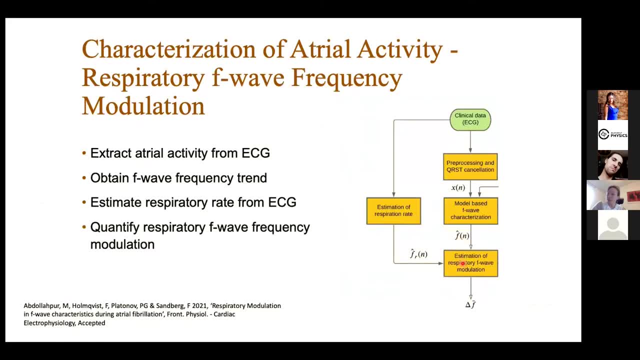 So there are other sources of variation as well, But we are interested in the ones related to respiratory modulation. So what we do is that we filter this frequency trend in In an interval That is defined by the respiration rate, And in order to do that, we need to know the respiration rate. 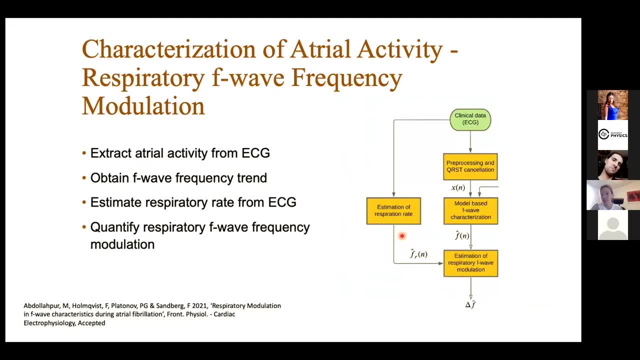 And in general. in this case, we don't have access to the respiration signal, So this method is only based on the ECG. That means that we need to estimate the respiration rate from the ECG, And we can do that. 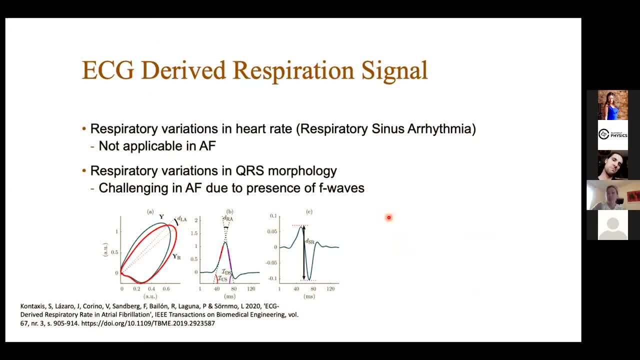 There are several methods available for ECG derived respiration. Quite common is to look at respiration respiratory variations, in heart rate, So this is called respiratory sinus arrhythmia. Basically, the heart rate increases with inhalation and decreases with exhalation. 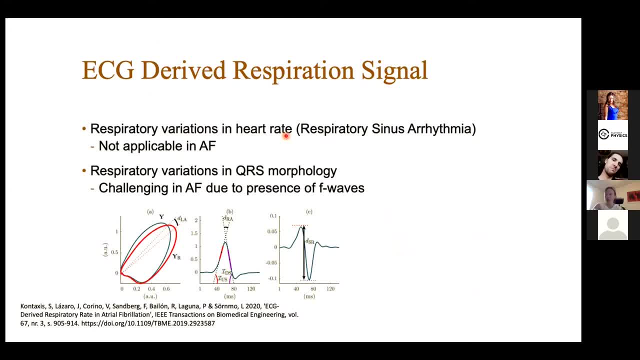 So, looking at variations in heart rate, we can estimate in general, we can estimate the respiration rate. However, this is not applicable in atrial fibrillation, Because the heart rate in atrial fibrillation is not determined by the rate initiated by the sinus node. 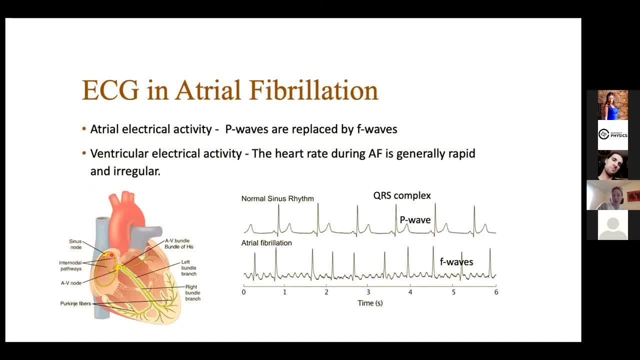 So, if you remember, In normal heart rate each heartbeat is initiated from the sinus node, But in atrial fibrillation we have a totally irregular and chaotic electrical activity in the atria And the heart rate is mainly determined by By those impulses that are conducted through the AV node. 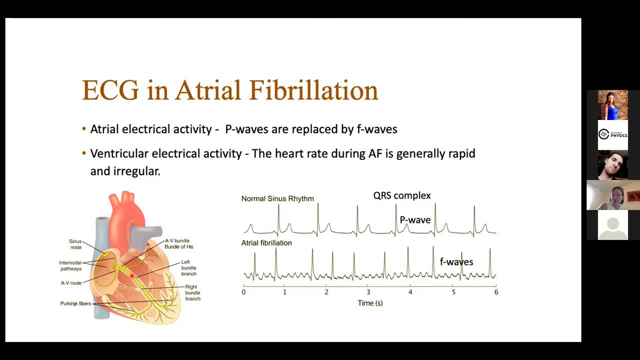 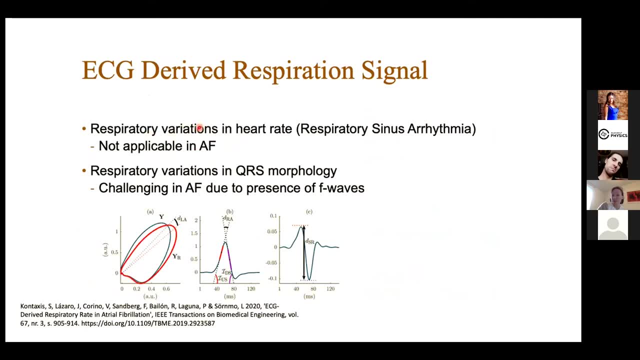 So there is a different mechanism for the heart rate during atrial fibrillation And therefore we cannot use this methodology to estimate respiration rate. But we can look at variations in QRS morphology. So, due to chest movements, The electrical axis of the ECG will change with the respiratory movement. 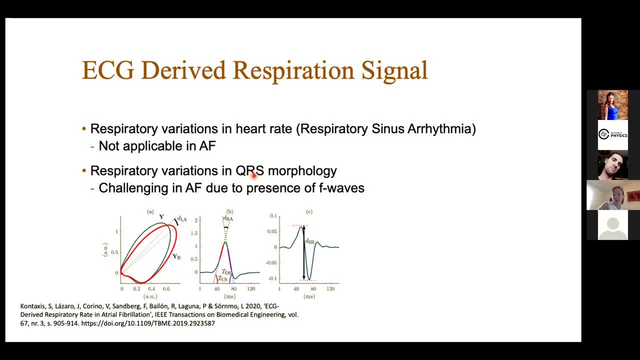 So there are several methods that are proposed to analyze this- respiratory variations in QRS morphology- And this works, but it's a bit more challenging in atrial fibrillation than in normal sinus rhythm Because we have the F waves that are overlapping the QRS complex. 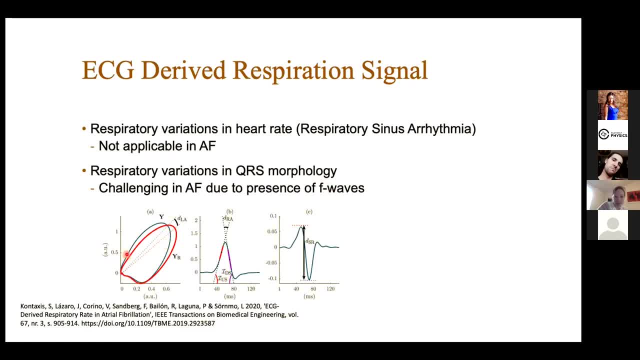 So these are some examples. This is, for example, looking at the QRS loop. So if we project the 12 lead ECG to the three orthogonal leads And look at a loop formed by the propagation in these leads, We can see that the loop angle varies with the respiratory cycle. 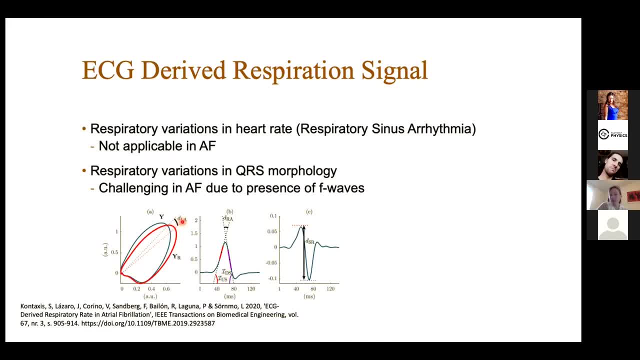 And this is information that can be used to extract respiratory variations and estimate respiration rate. Another approach is to look at the angles of the QRS slope, And yet another here is to look at the first derivative of the ECG And also quantify the slope. 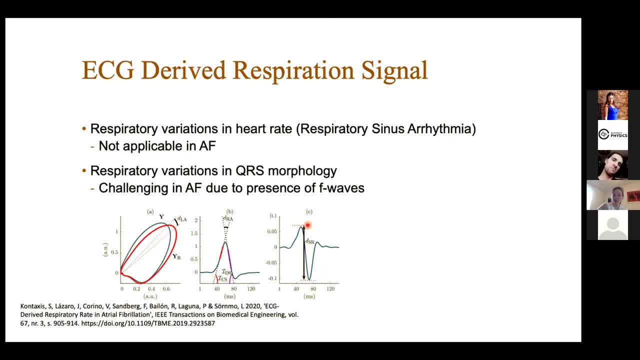 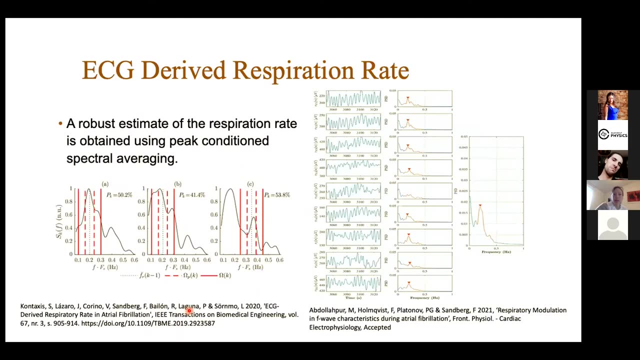 The slope range here Between the maximum and minimum slope, And this is actually the method that was shown to be more robust in the presence of F waves during atrial fibrillation In this work. Okay, so we estimate this respiration signal separately for each lead of the ECG. 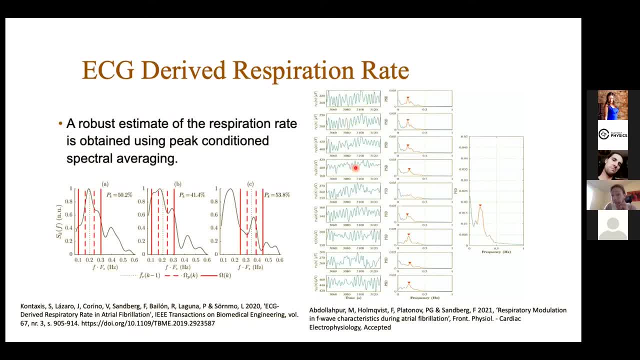 So this is the extracted respiration signal- One example here- And then from each of these signals, from each lead, we obtain a spectrogram, And then we average only those that are of sufficient quality. So this is similar to the method that I used to estimate respiration rate in hemodialysis. 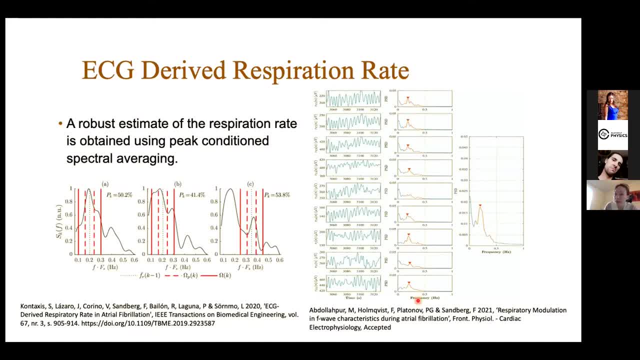 We have a quality control of the spectrum And then we average the spectrum from which we can estimate a more reliable respiration rate, And the criteria for deciding if a spectrum is of sufficient quality is basically that we have a peak in the respiratory interval. 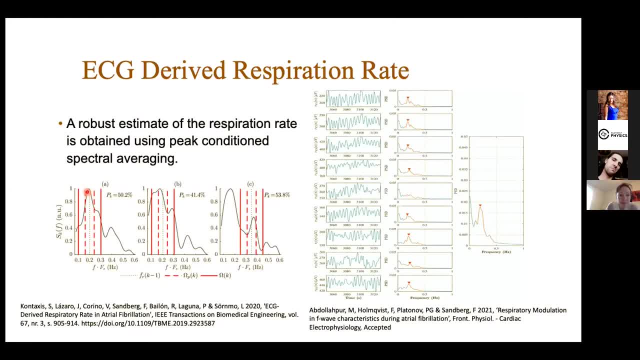 So this interval here Which is defined based on The previous estimated respiration rate, So the respiration rate in previous time segments, If there is a sufficiently large peak in that area, we say that the spectrum is of sufficient quality And it's contributing to the average. 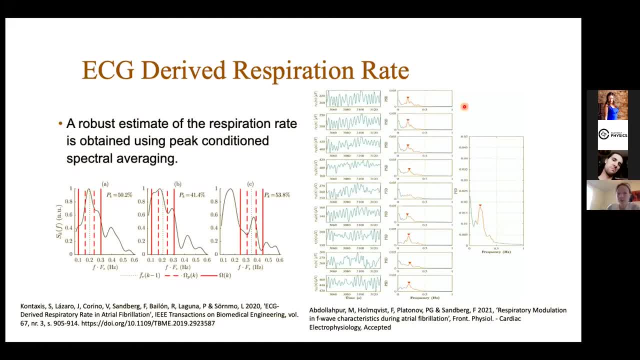 From which we estimate the respiration rate. So in this example, this is a sufficiently good spectrum. This is not sufficiently good Because there is not a sufficiently large peak in the respiratory interval. And the same for this: There is a peak in the respiratory interval, but it's not sufficiently large. 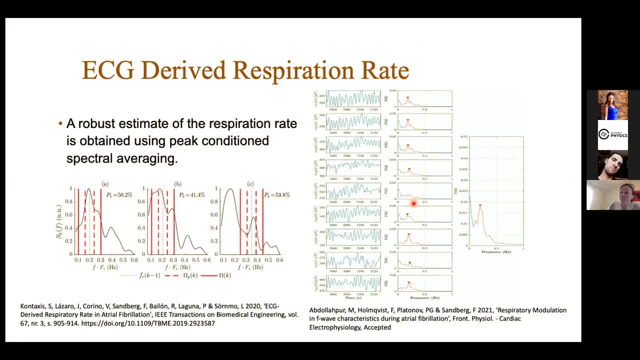 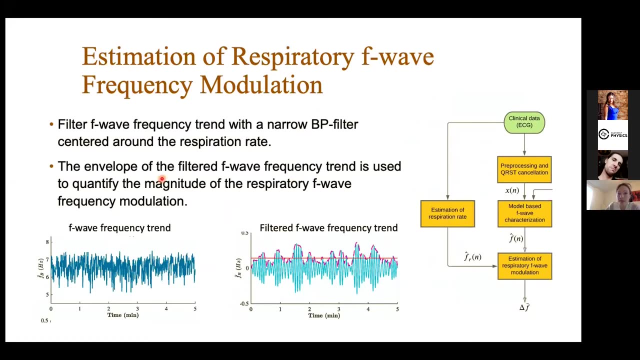 So it's peak condition spectral averaging, basically, that we use to estimate the respiration rate. Okay, So once we have the respiration rate, we filter the F-wave frequency trend in a narrow band around this respiration rate. So this is the F-wave frequency trend that I showed before. 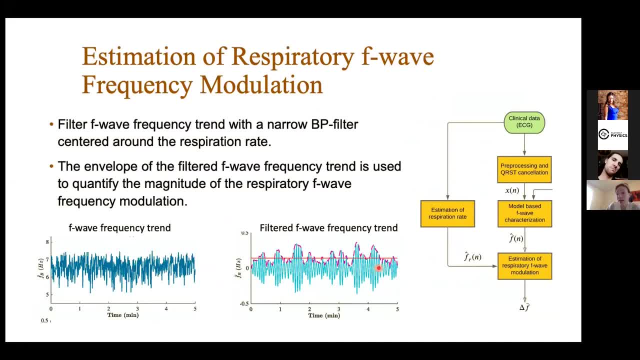 And this is a filtered F-wave frequency trend in the respiratory interval And then we look at the magnitude of this filtered, Filtered F-wave frequency trend And we use that to quantify the magnitude of respiratory F-wave frequency modulation. So this is. it varies quite a lot over time. 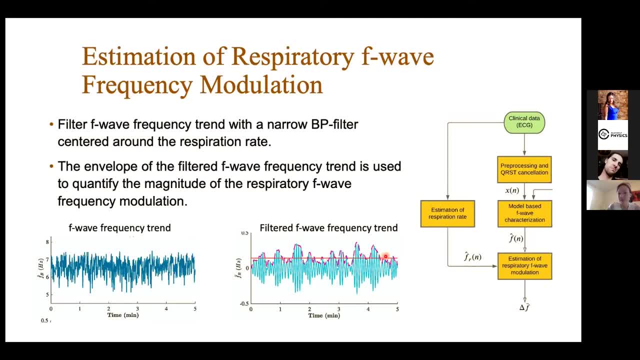 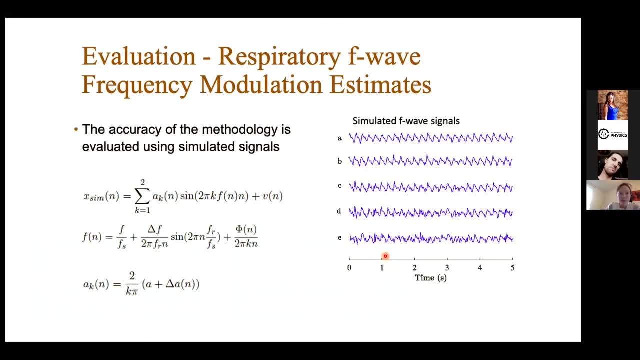 But this is the average in the five-minute segment that we apply. So this method was evaluated with a series of tests And we simulated F-wave signals. So this is a model which we use to simulate the signals. It's basically a sinusoidal model. 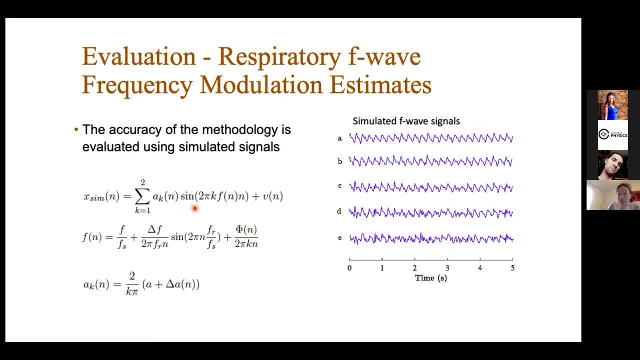 Sum of two sinusoids, The sinusoid and its harmonic, And it has a varying, time-varying amplitude. It has a time-varying frequency and additive white noise And the time-varying frequency is dependent on. So there is a baseline frequency. 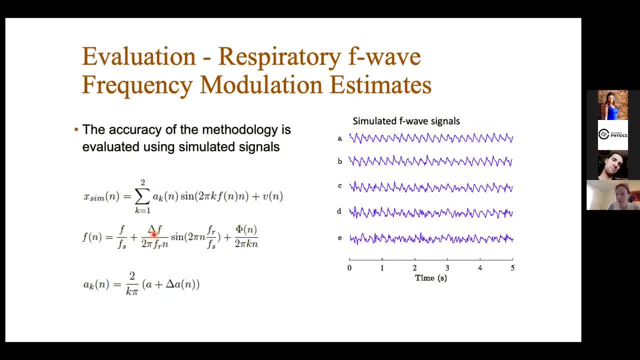 Then there is respiratory modulation And then there is random phase variation, Accounting for other types of frequency variations, And we can see that the signal quality index- That is the fit of this model, The model signal that I showed before- The signal quality index is decreasing the more random variation we have. 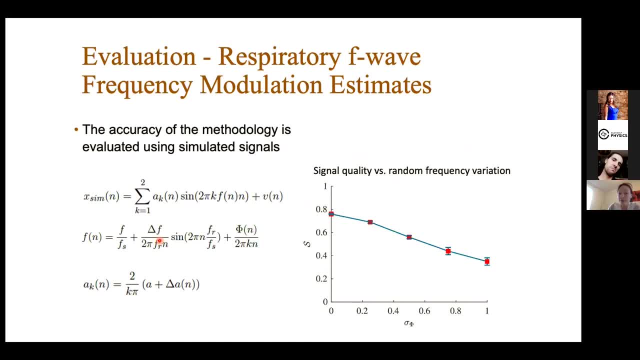 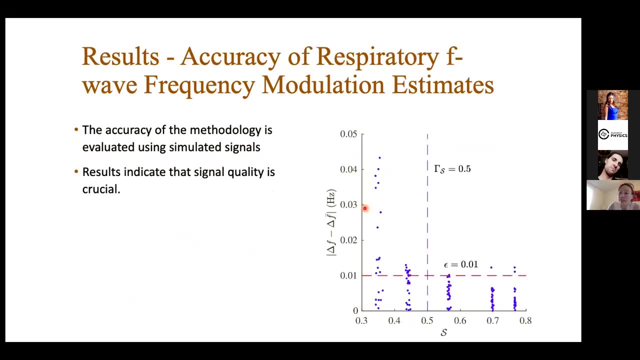 So that means that the estimate, When we try to estimate the local frequency, The estimate will be less reliable the more random variation we have, Which is natural. And looking at the methodology for extracting the respiratory F-wave frequency modulation, We can see that if we get a signal quality index, 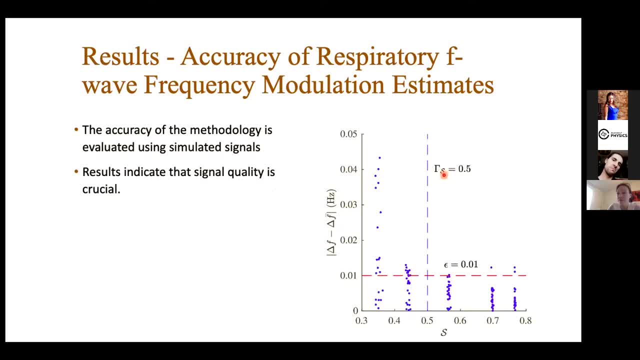 So, based on this- A large set of simulated signals With the methodology I showed before, We see that if we have a signal quality index above 0.5. We can get an accurate estimate Of the magnitude of the respiratory frequency modulation. 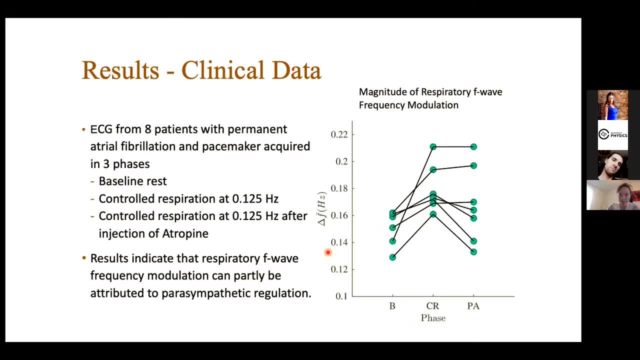 And This is an example. This is: We applied this to clinical data From eight patients with pacemakers in permanent atrial fibrillation And They had also a pacemaker And they were in a clinical trial Where they were in. 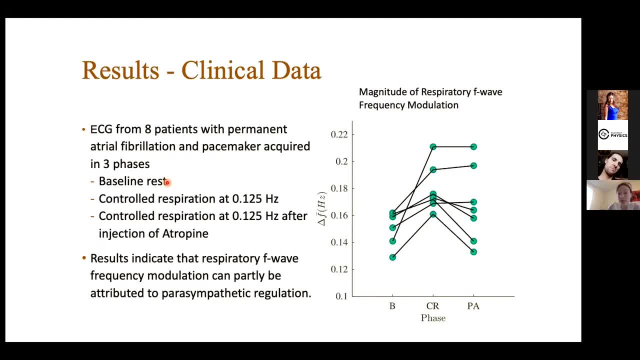 ECG was recorded in three phases: Baseline rest And then they were asked to breathe at a frequency of 0.125 hertz. And then they were asked to breathe at The same frequency And they got an injection of atropine. 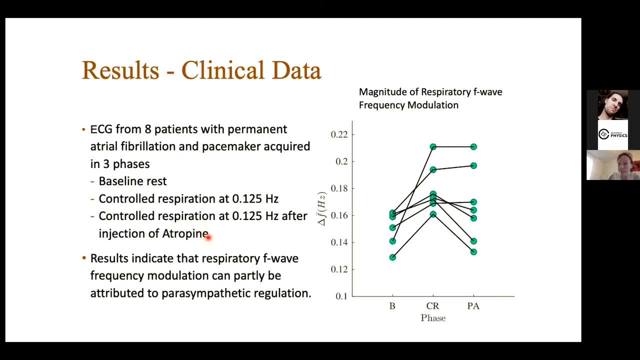 Which is a blocker of the parasympathetic activity. So it's blocking parasympathetic regulation, basically, And what we can see here is that the magnitude of respiratory frequency modulation: It increases When the patients are breathing Slowly. 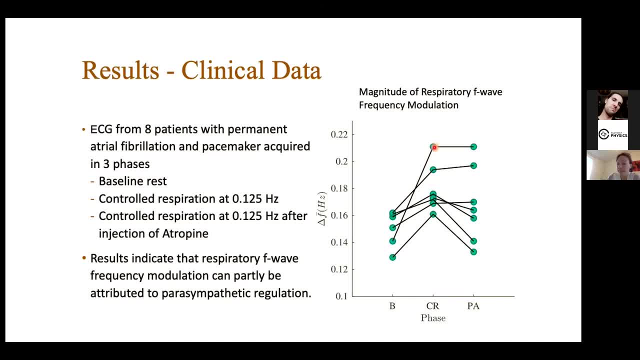 Deeply, Which is expected, Because with deep breathing we get an increase of parasympathetic regulation. And then we also can see that After injection of atropine, In some- Approximately half- the patients There is a decrease in the magnitude of the respiratory modulation. 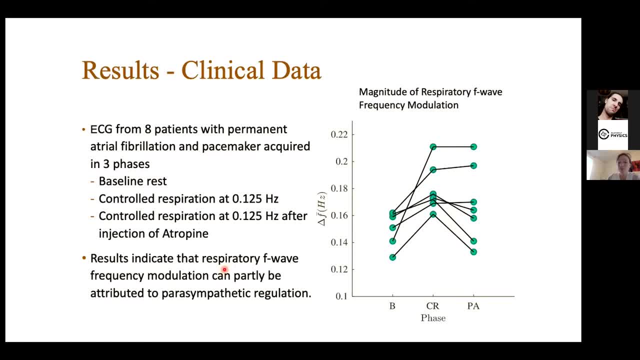 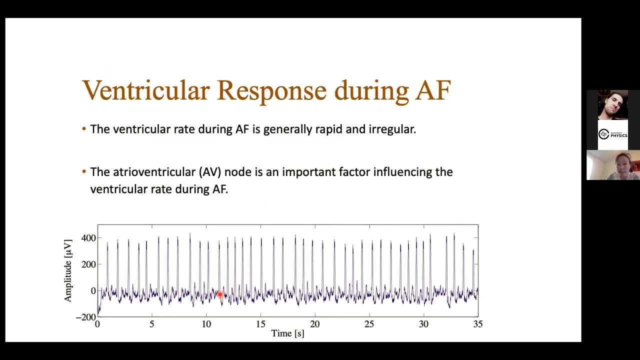 However not in all patients. So from this we can see that respiratory F wave frequency modulation Is partly attributed to parasympathetic regulation. I can see that I'm running out of time, So I'll go through this last example really quickly. 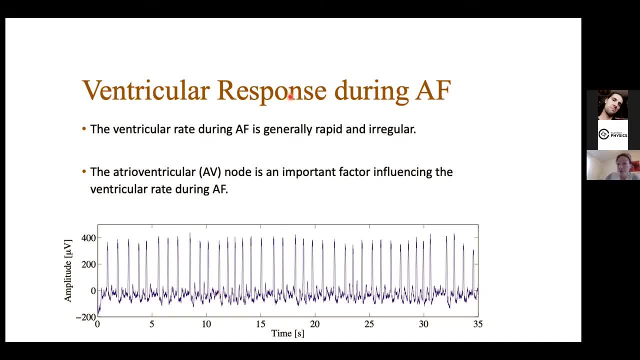 So, as I said before, Ventricular response during atrial fibrillation is rapid and irregular And the AV node, That's electrical Point of conduction between the atria and ventricle, Is very important in regulating the ventricular rate during atrial fibrillation. 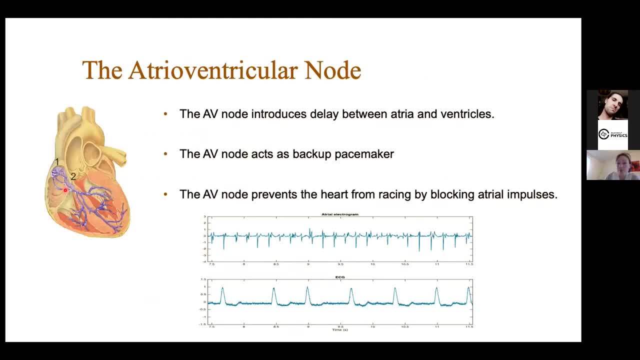 So basically the purpose of the AV node During atrial, During normal sinus rhythm, Is mainly to delay conduction between atria and ventricles, To allow filling of the ventricles, And it can also act as a backup pacemaker. 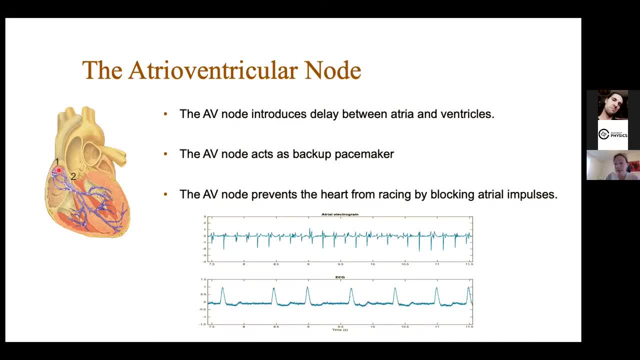 If the sinus node fails, There is. It can induce Heartbeat From the AV node, But during atrial fibrillation The most important Function of the AV node Is to block atrial impulses And prevent the heart from racing. 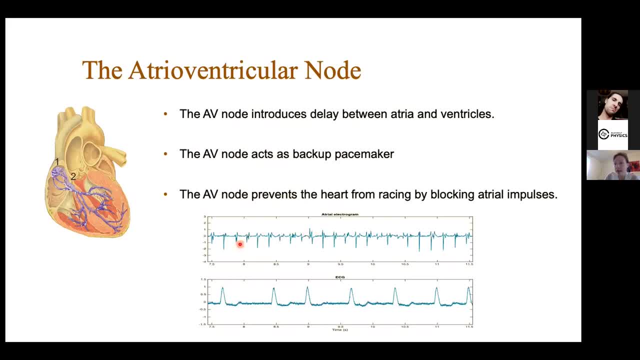 So this is an example. here Is an intra atrial electrogram, So you can see the atrial impulses Here close to the AV node, And this is a corresponding ECG And, as you can see, Several of the atrial impulses. 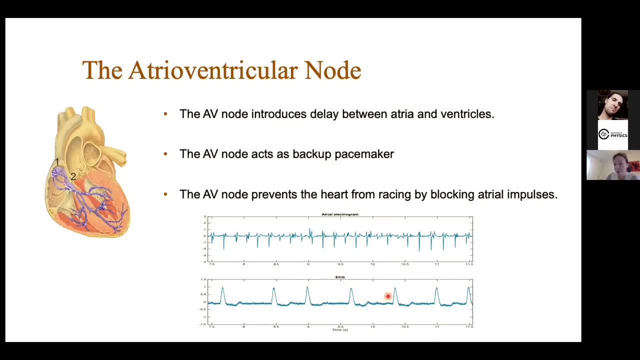 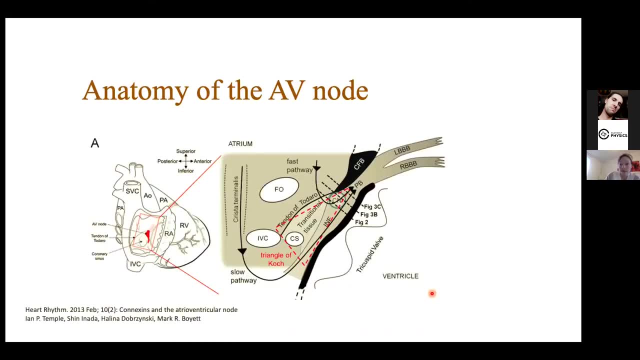 Are blocked And only A fraction of them Will actually result in A ventricular activation. So the AV node: basically It's a complex structure, But one important Property Is that it has a fast pathway And a slow pathway. 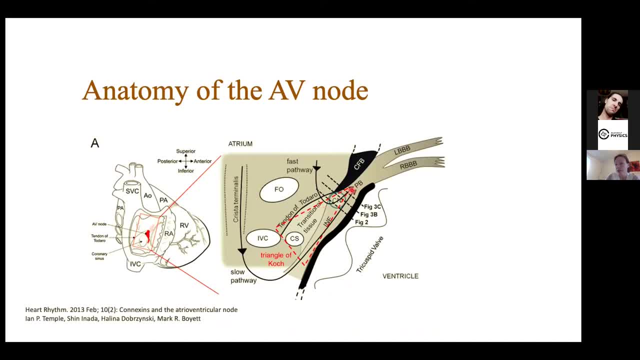 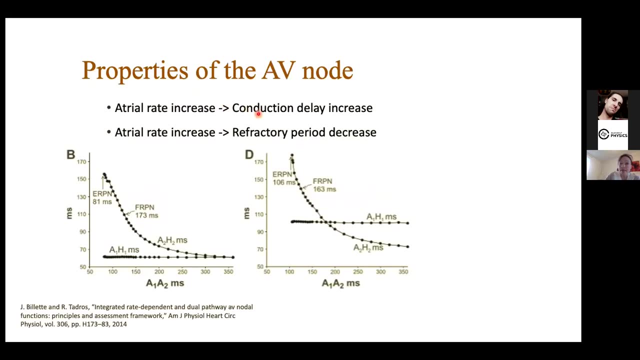 So fast pathway With Faster conduction But longer refractory period, And the slow pathway With Slower conduction But Shorter refractory period, And So we have the Conduction delay In the AV node. 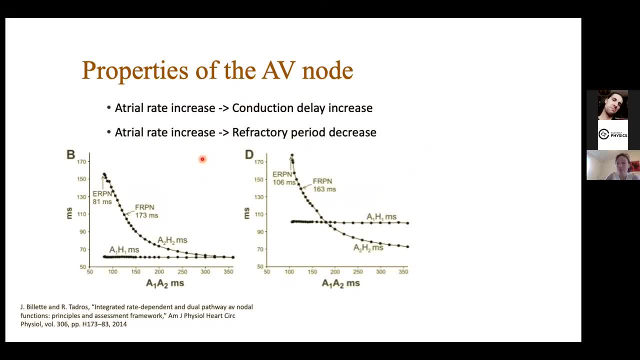 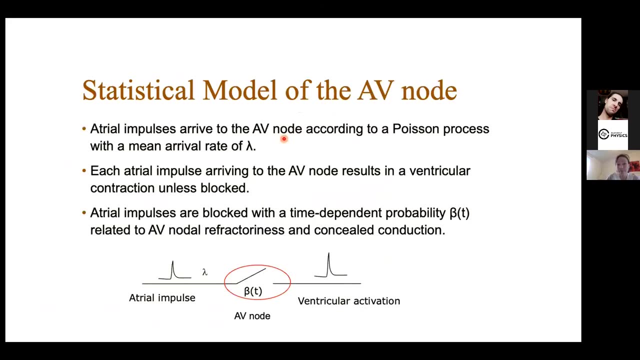 And we have the refractory period And these are both Rate dependent. So if we have, You can see by pacing experiments: If the atrial rate increases, The conduction delay Increases, And if atrial rate increases, The refractory period decreases. 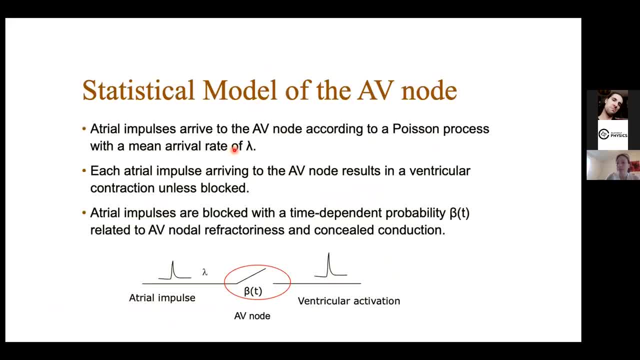 So it's quite a complex structure And we wanted to model this In a simplified way To be able to extract Important information From the ECG. So basically, in this Statistical model We assume that Atrial impulses arrive. 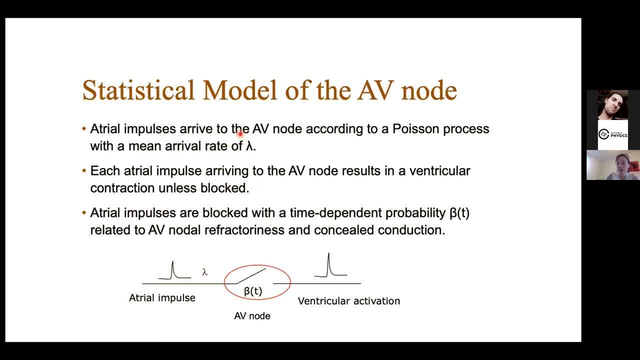 To the AV node According to Poisson process, With some mean arrival rate, And this mean Arrival rate Is estimated From the F waves Of the ECG. And then The AV node blocks Some of the impulses And 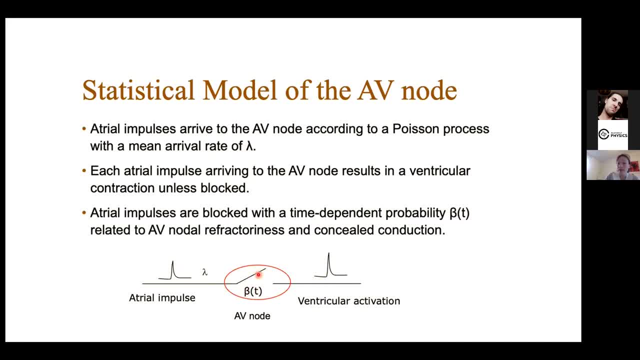 And it conducts Some of the impulses, And The probability Of blocking Is Time dependent. So this, This blocking probability, Is related to AV node refractoriness And also Concealed Conductions. It's related to the 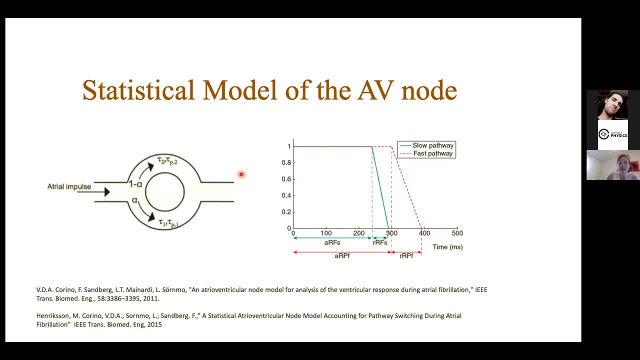 History of Impulses And, as I said, This is a Very simplified Model. So, basically, We assume that An atrial impulse Can take Either the Fast pathway Or the slow pathway And the probability Of blocking 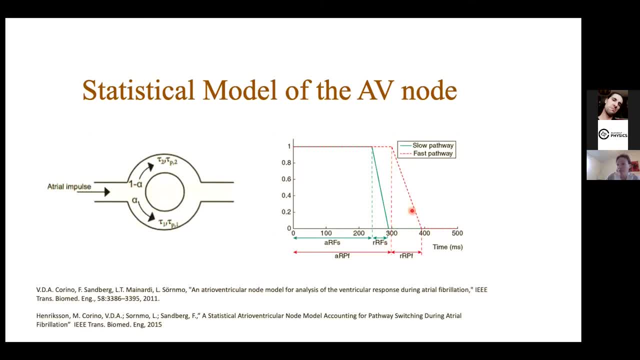 Is time dependent, As I said before, And it's different Between these two pathways. So basically, After a certain time Since the previous Ventricular activation, All impulses Are blocked, And then After An extended Time period. 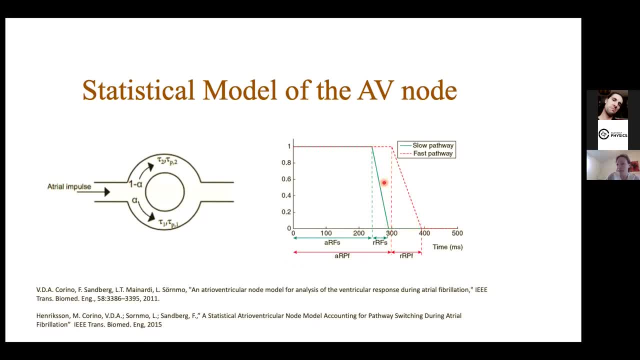 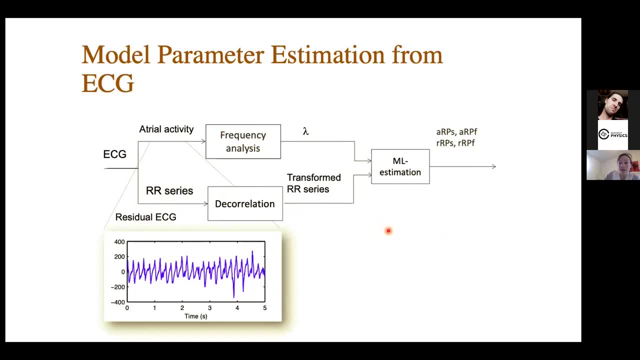 Not No impulses Are blocked And between These two, The probability Of an impulse Being blocked Is linearly Decreasing. So We can estimate This model Parameters Related To the Blocking From the ECG. 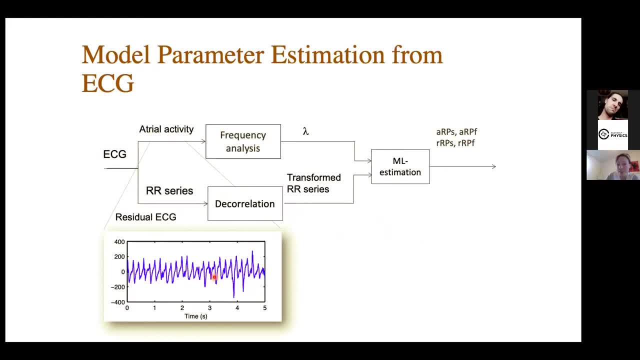 Basically, We have the ECG, Then we have the Atrial activity, The F waves, And we do, We analyze The frequency Of this, The Frequency Which is Assumed to be The arrival rate Of the 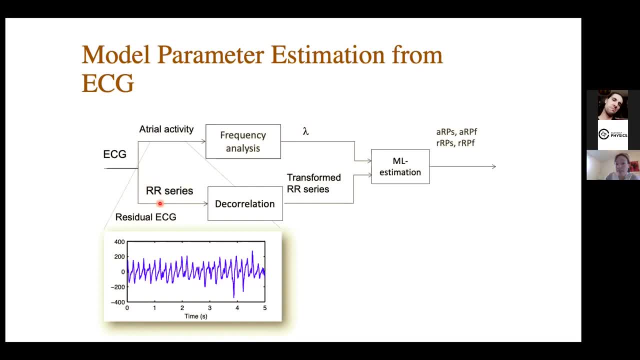 Atrial impulses To the AV node. Then we got The RR interval Series, The series Of ventricular Activations, And we Do some Correlation Because we Need to assume That the Ventricular 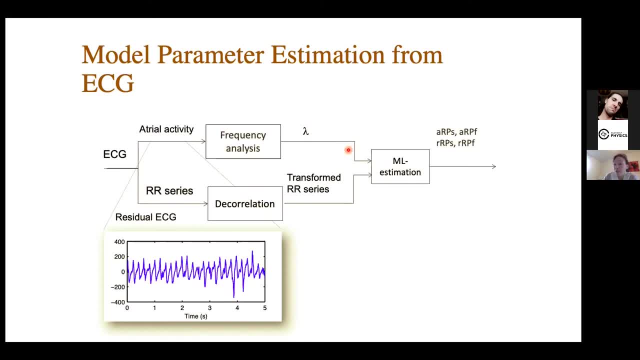 Activations Are independent And then, Based on The Assumption That we have That the Output Is, Or the Probability Of blocking Result In this RR series, We can apply Maximum Likelihood. 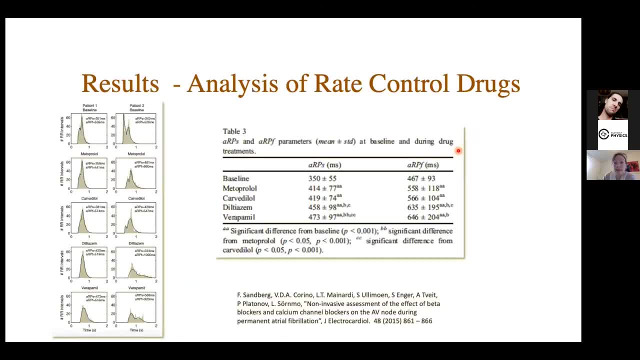 Estimation To Obtain Model Parameter Estimates, And We Did This. This Is An Example Where Applied This Methodology And We Did Assess The Effect Of. 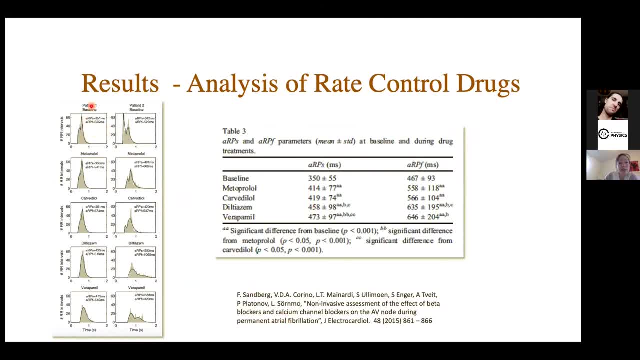 Beta Blockers And Calcium Channel Blockers. So Here On The Left Hand Side, There You Can See The RR Interval Histogram. For The Interval Histogram. 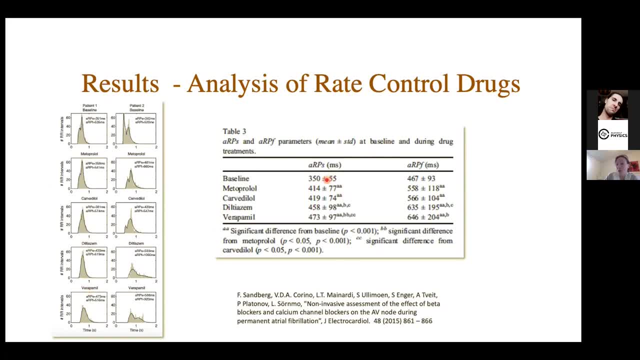 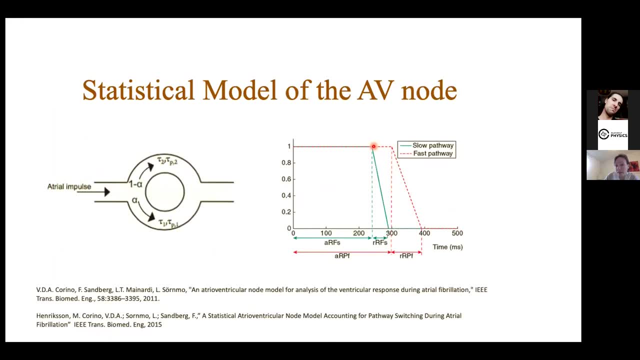 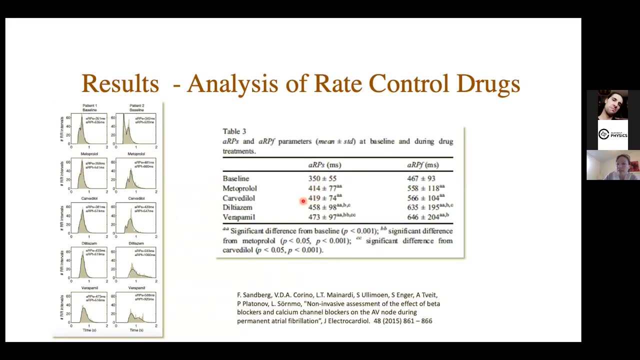 Changes With The Treatment And We Can Also See That The Model Parameters Here Related To The Absolute Refractoriness Which Is This Time Point. 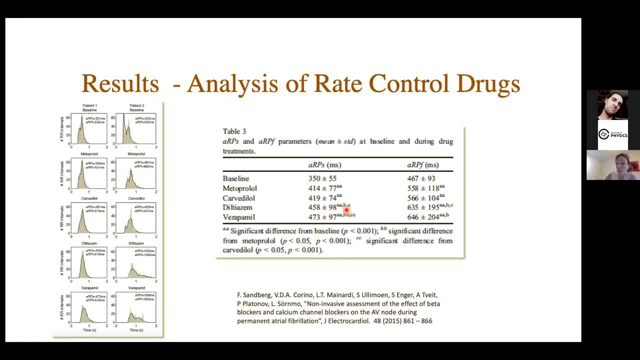 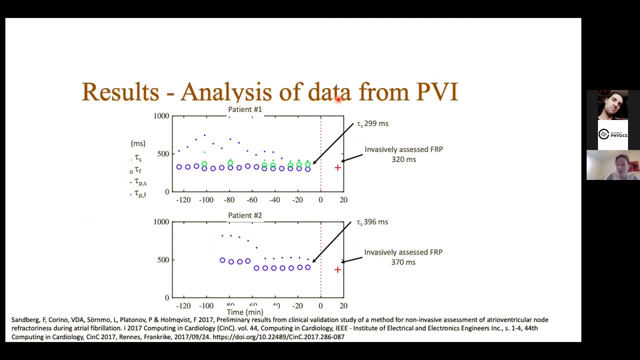 This Time Point, This Is More For The Calcium Channel Blockers Than For The Beta Blockers. And Finally, We Tried This Method To Analyze. 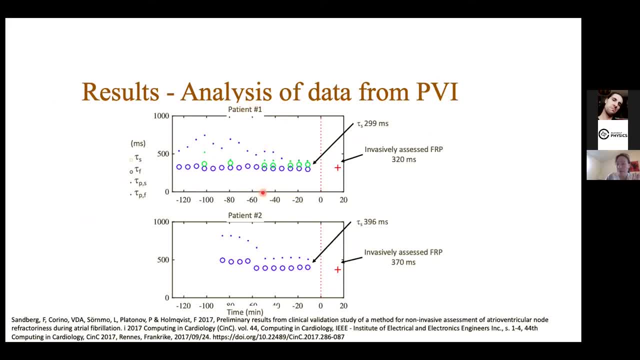 Data From Pulmonary Vein Isolation So Obtained During Analyze, The ECG Signal Prior To This PVI Treatment. So Catheter Ablation Where. 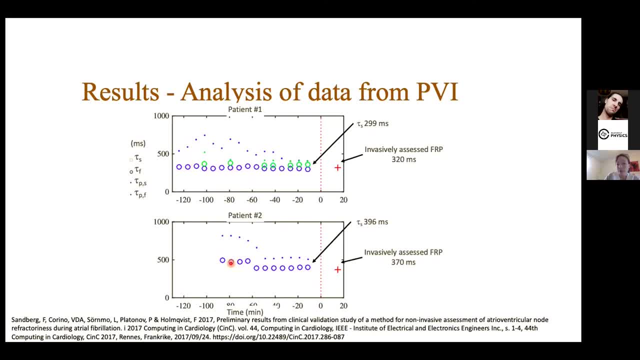 They, They Go In And Burn Around The Pulmonary Veins To Stop The Fibrillation. So Here, Once You Are In Sinus Rhythm, We 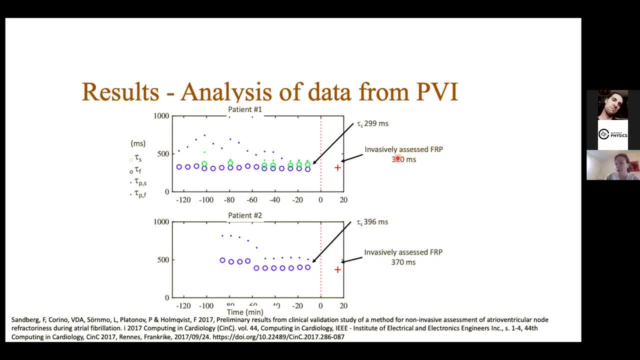 Can Run A Pacing Protocol To Assess The Functional Refractory Period Of The Node And We Compared This Functional Refractory Period To It. 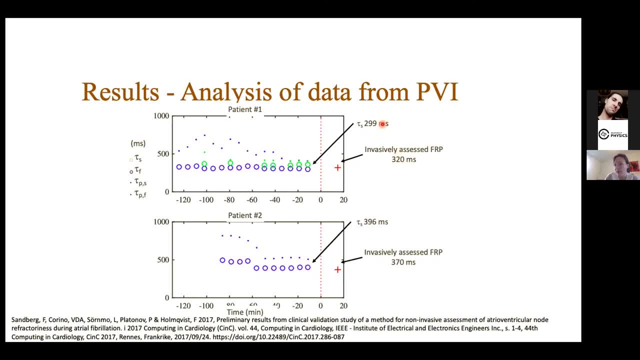 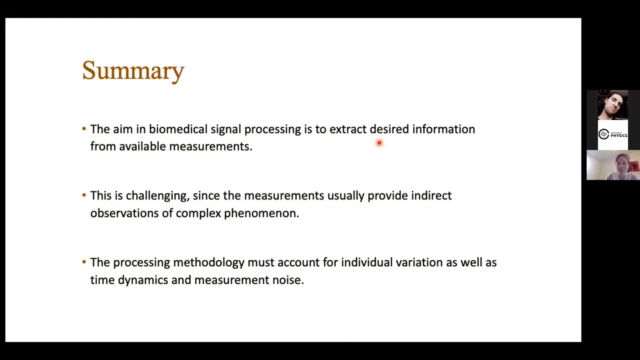 Would Be A Reasonable Result. So This Is We Can. Based On This Result, We Can Basically Say That Our Estimate From The ECG Is: 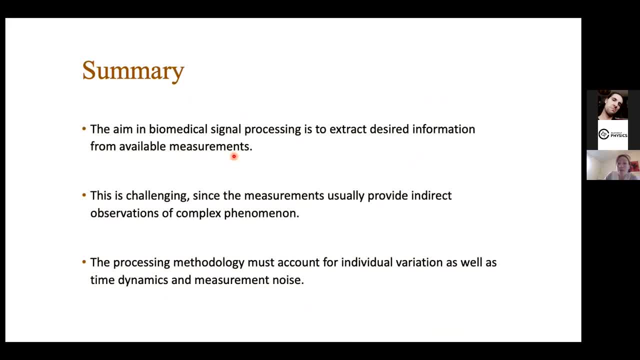 In Line With The Biological Processing Is To Extract Desired Information From Available Measurements. So Sometimes What's Desired Is Not Available. So And And This 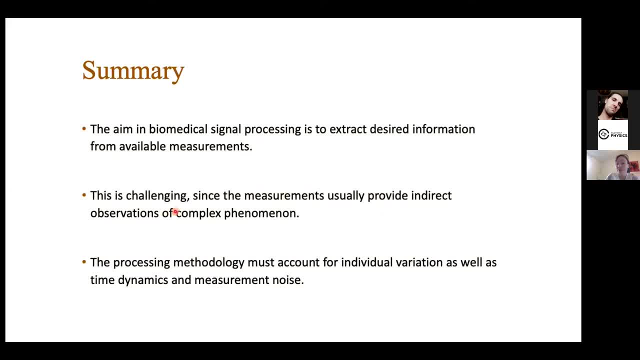 Is The Challenge. So Sometimes We Cannot Measure Directly Based On What We Know About The Physiology And What We Know About The Measurement And 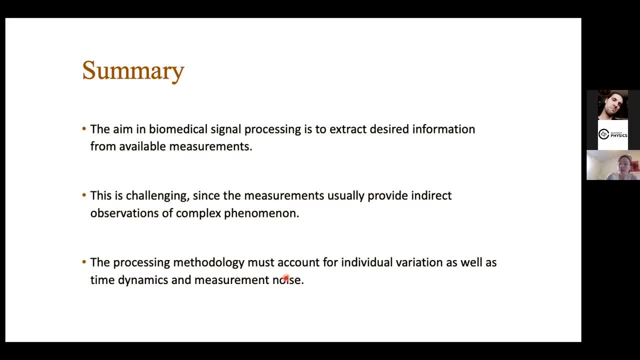 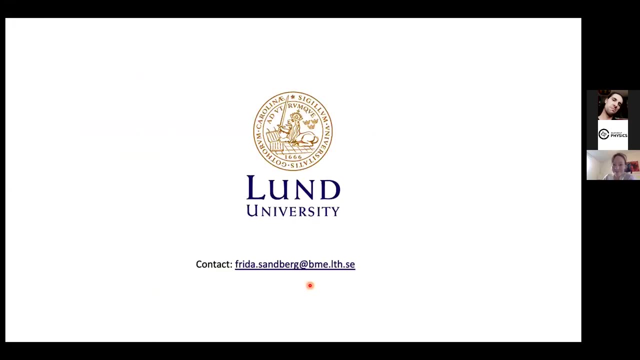 So On, And We Sometimes We Need To Use Some Modeling As Well, And So Thank You Very Much. Thank You, Frida, For The Interesting 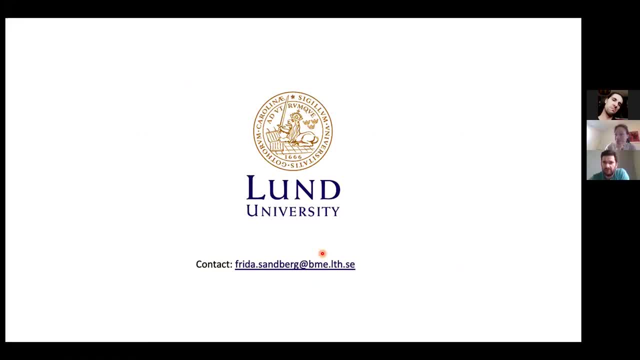 Talk. So, Dear Colleagues, Do Have Any Questions. So, Mikhail, Raise A Hand, Misha, Please. Okay, Thank You. So I We Do, M R. 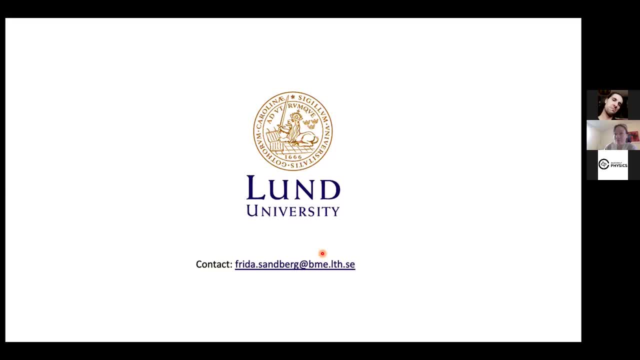 I And M R I, Particularly In Cardiac M R I There Is A Problem That With When There Is Arterial Fibrillation, The Heart 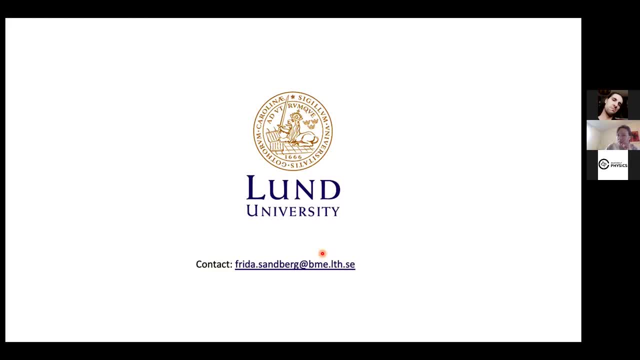 this is the moment where we can do scanning. so the problem is the ventricles doesn't contract. the ventricle don't contract, so the heart is pretty much stable and doesn't move. so we can do scanning, scanning in that period. but because of the heart rate is so irregular, it often happens. 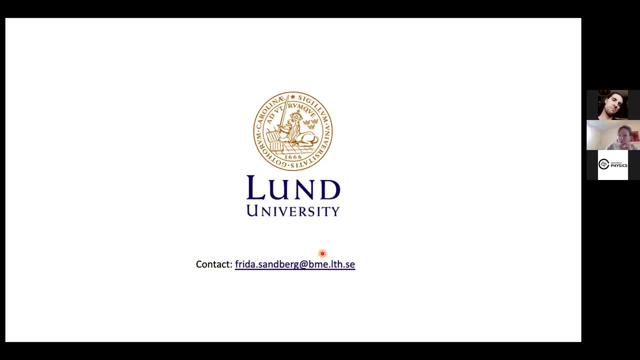 that when we assume there would be some vacant time for scanning, there is no because there is another qrs complex coming. so the question is: do you have some methods of, say, predicting the average available time after the qrs complex depend, maybe taking into account the shapes of the f waves or maybe the shape of the qrs complex to assess if there would? 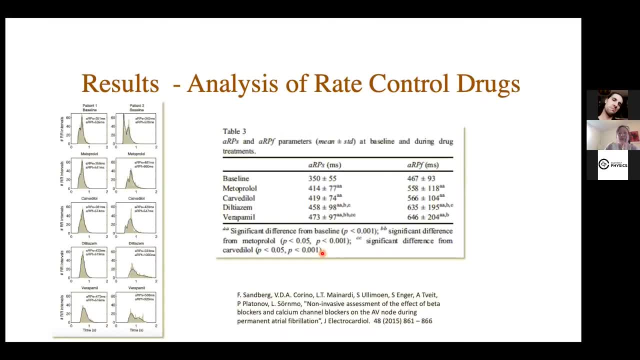 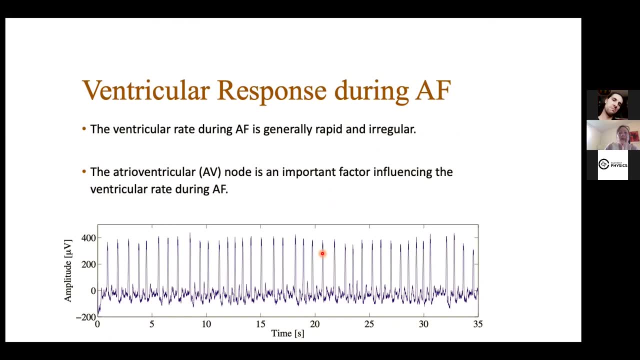 be enough time for a scan after, after a particular qrs complex and may probably do it in line when you actually do the scanning. so so that there is a decision process to do the scan or not to do the scan, right. i i think, um, it's not well, it's, it's somewhat related. 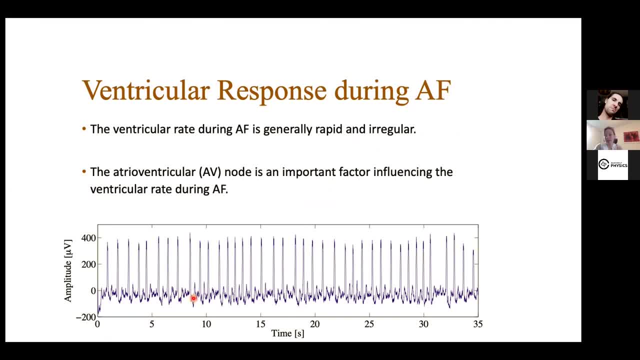 to the f wave characteristics because it's related to the um atrial fibrillatory rate. so f wave frequency, the faster f wave frequency indicates that you have more impulses arriving today. so on the Hillitin type, we have a lot of people in the hospital saying 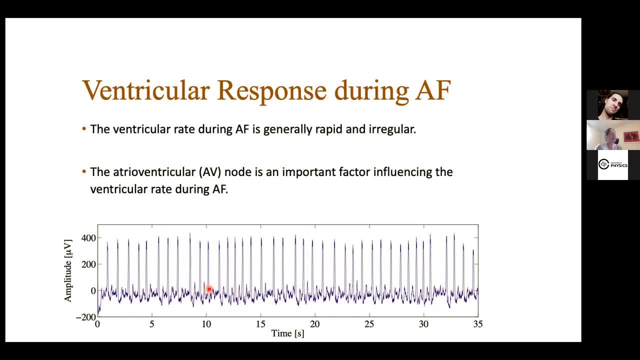 that i, you know, i'm having very high rt iste males and on my quad as well. i know the herps side, that's what it is. but so to the qrs complex neighbours that i always gave a note, and probably i mean that that is related to to the generation of ventricular activations, but the qrs complex morphology, i don't think that would affect it. i think probably the best would be to have a model, so based on the history of rr intervals for that specific patient, you could probably make a prediction on the child. 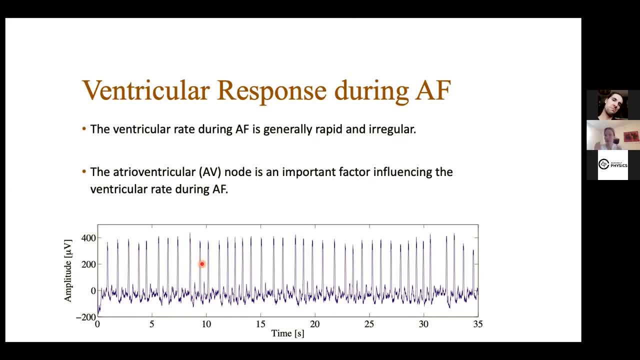 on on the um, like the time interval between between consecutive activations in like i mean, that would be something interesting to try out at some point probably. if we encounter that, i probably would email you with some details with that. okay, thank you, that's really interesting. yeah, thank you, michi. so we have a question from the chat? uh, yes, 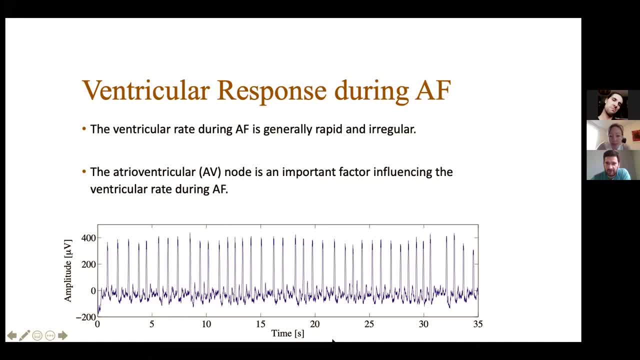 okay, a lot of questions, so i can read it, or: uh, yes, let me see. i i think i got the chat here. uh, in the part where you characterize f waves, do you account for some other diseases in addition to atrial fibrillation? I wonder what will be the result of the characterization of a patient who 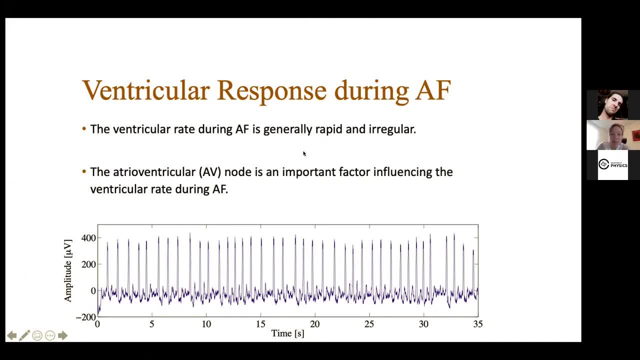 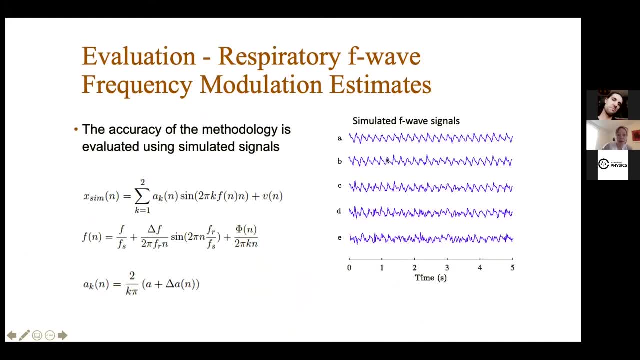 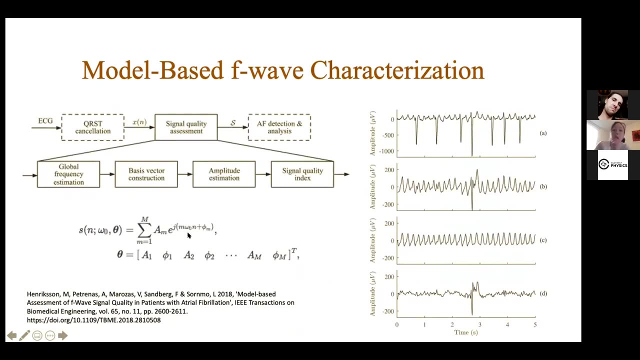 has some pathology which can't be fitted by the analytic model. Yes, so in the characterization of the f waves. basically here I mean this model. in my experience- and I have analyzed quite a lot of f wave signals- this type of model like a harmonic sinusoidal model, in this case a 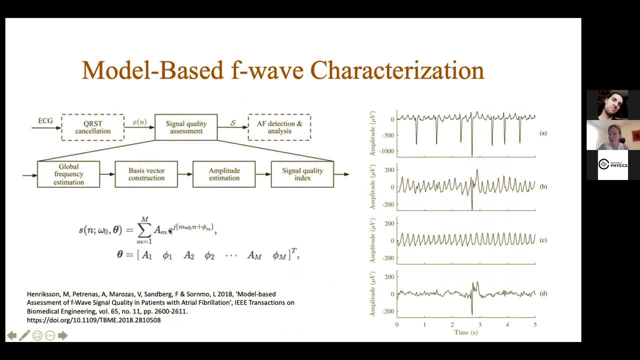 complex sinusoidal model. it generally fits quite good. It can describe the f waves in most of the cases. Other pathologies- I mean yes, there could be other pathologies- Do you mean pathologies in the f, in the atrial activation pattern, or pathologies in general? 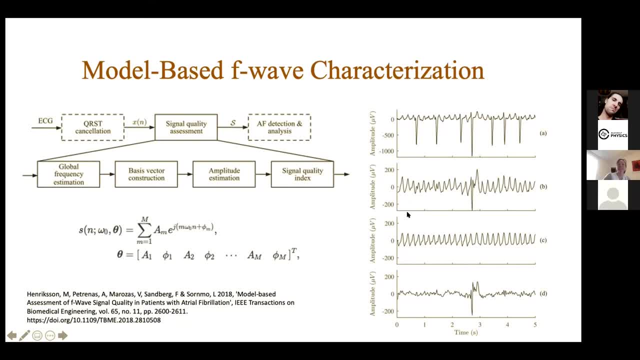 Hello, pathologies in general. Pathologies in general. Pathologies in general, Okay, I mean if it's pathologies related to, for example, if it's a patient that has a lot of ectopic beats, of course the QRS decancellation will be more difficult. So 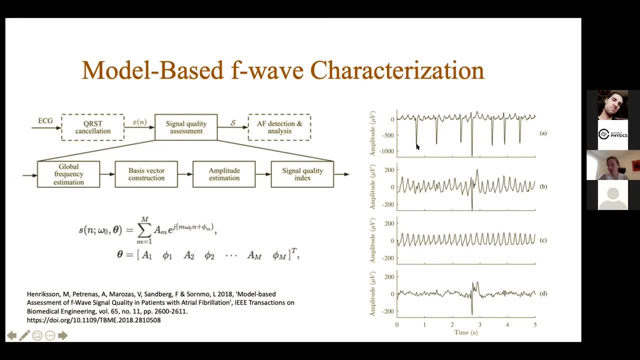 if you have a like. if the QRS complexes looks will be very different, then of course they will. the QRS decancellation would be more challenging, But I mean, that's a different thing Also. so the f waves can look quite different In this case. in this example they are. they're quite 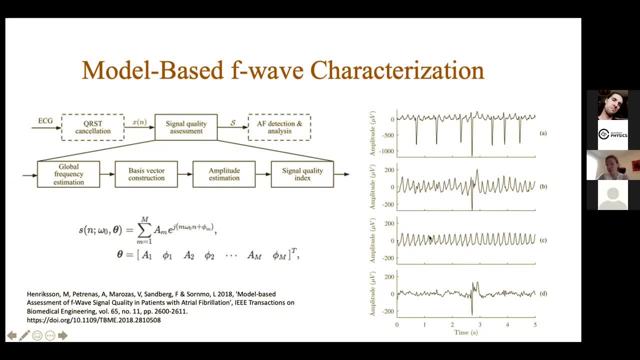 large amplitude and quite regular. but they can also be with a small amplitude and fairly irregular. So for example with patients with heart failure, they often have quite a low amplitude of the f waves and low frequency and quite chaotic behavior. So they can look very different. But 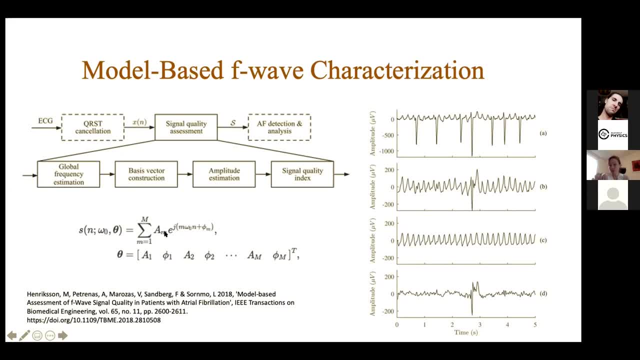 Fitting this type of model to a very short time segments generally works quite accurately, I would say, even with other pathologies. Okay, thank you. Okay, do you have any other questions? Okay, so maybe I have one, maybe a little bit stupid question, but so it's regarding the atrial fibrillation. 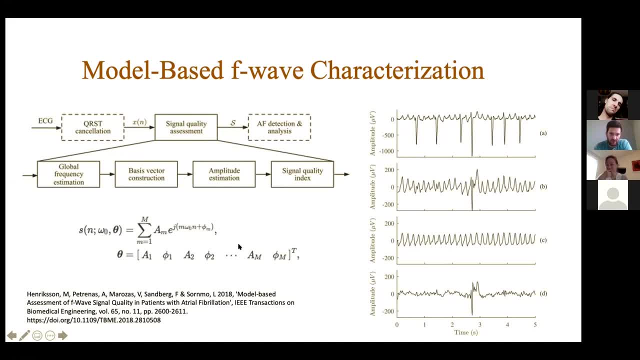 So you have some analysis for this spectrum and what's next? Can the doctor use your analysis and your information to heal the patient or to do with Yes? I mean, we don't know that yet because first of all, we need to be able to measure it and, as you've seen, it's quite complex to extract this information. 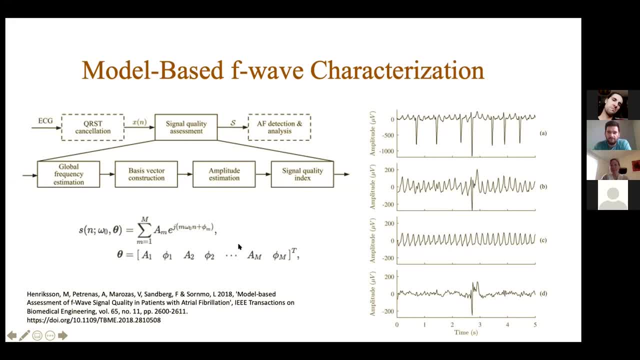 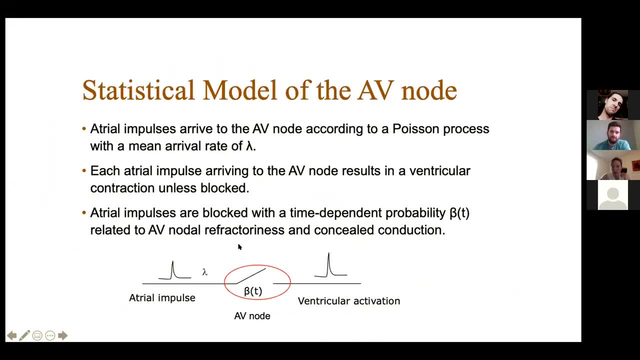 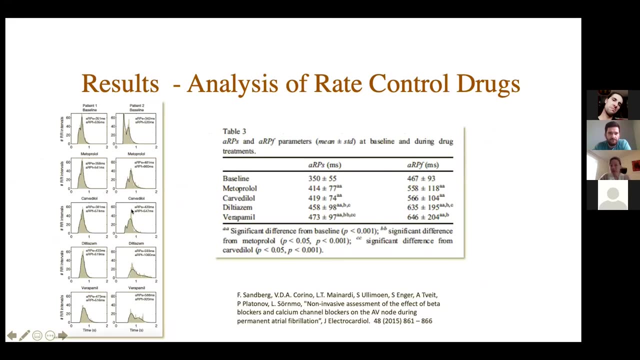 Then we need to show that this information is actually useful. So, for example as a case with With that AV node model, We could Apply it to analyze the effect of various drugs. So this is a type of application that we could also see. how would, for example, drugs affect the respiratory F wave modulation? 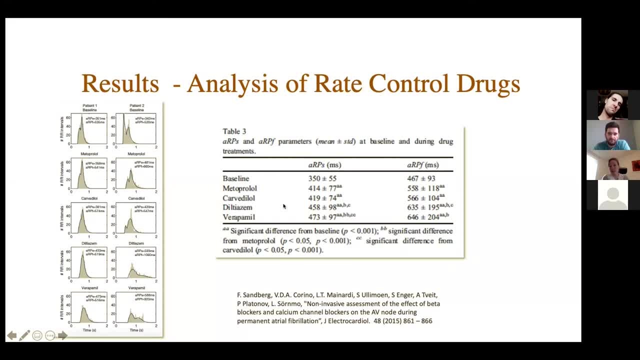 But I think even more interesting when it comes to respiratory F wave modulation would be the relation between that and disease progression. So I believe that this is related to disease progression and with the progression of atrial fibrillation it's generally more difficult to convert to cardiovert, or the success rate of pulmonary vein isolation is lower. So 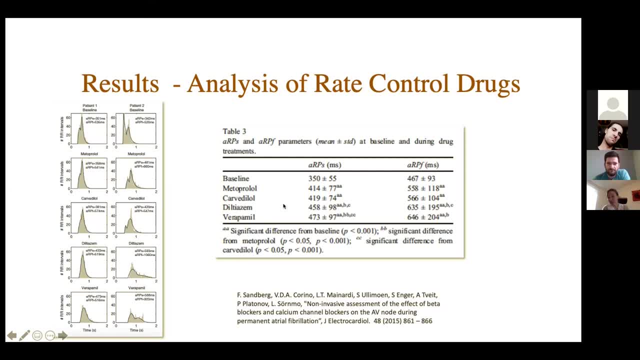 If we could extract that type of information that could be useful in the future as decision support for which, For which treatment to select for which patient. Thank you, And are you working with some medical centers regarding these problems? Yes, yes, yes, I work quite a lot with the. 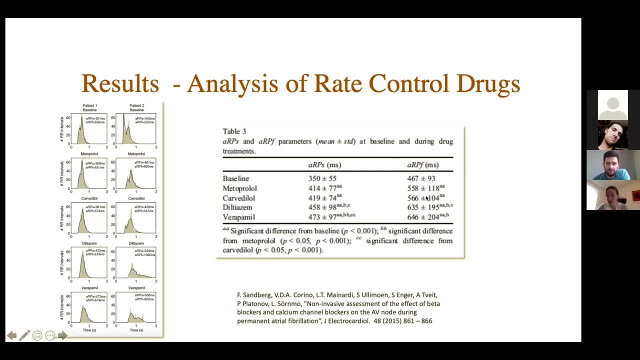 electrocardiology department in a hospital in Lund, but also- I mean in this case it's a group in Oslo in Norway. but I've also worked with some doctors outside Milan In hospital there and also outside Bologna. So there are. 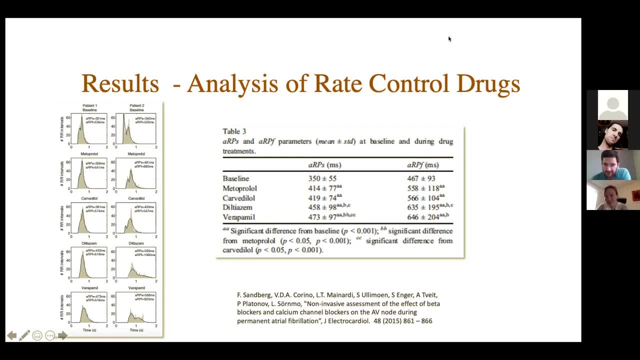 Okay, thank you very much, And Maria Grashko raised her hand. So, Marisa, Yes, I would like to ask: when you estimate a respiratory rate from ACG, is it possible to estimate a respiratory phase in addition to it? I mean to distinguish between inhale and exhale. 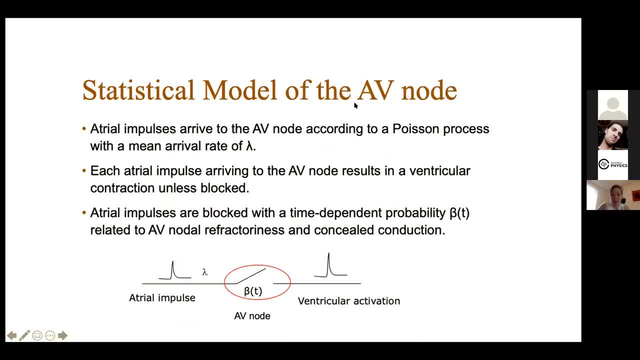 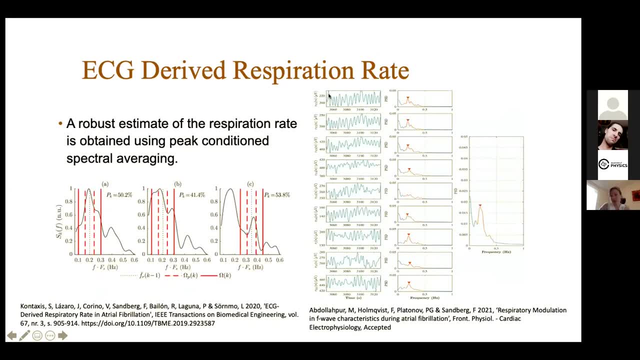 It is, but it's more, it's more challenging. So I mean Yeah here. So this is the extracted respiratory signals, right? so from each, each lead. So this: based on these signals, we can actually estimate if it's inhalation or exhalation. 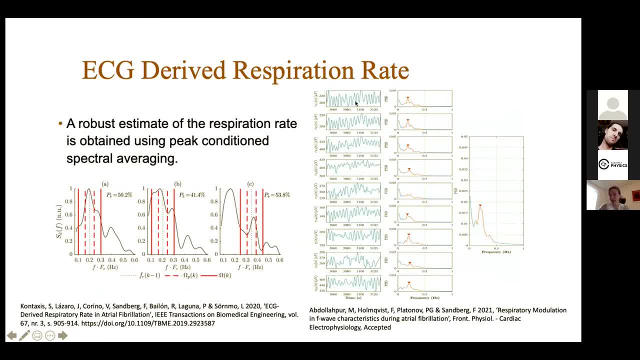 So it is possible to do that, but it's more, It's less robust than to just estimate the average rate. So I mean, if Yeah, it depends on what, what you need, but it is possible to do it, Thank you. 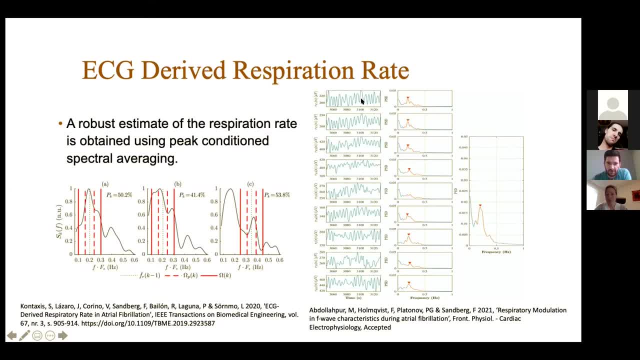